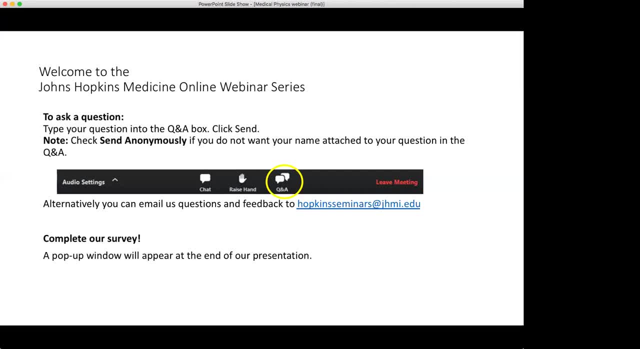 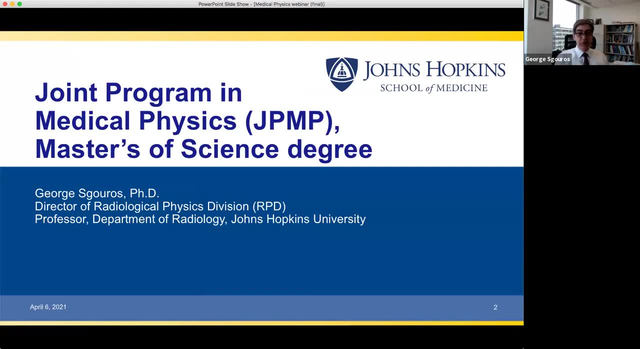 And now I would like to welcome Dr Segores to begin our presentation. Thank you, Amy, and thanks to everyone for attending. I'm absolutely delighted at the opportunity to share with you some information about our new master's in medical physics program here at Johns Hopkins University in Baltimore, Maryland. 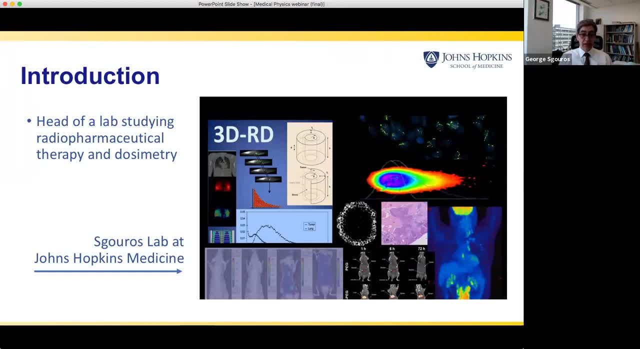 So, just by way of introduction, I'm the head of the radiological physics division and also the head of a lab, And also the head of a lab involved particularly in radiopharmaceutical therapy and dosimetry, And what you see on the screen are just some examples of some of the work we do in the lab. 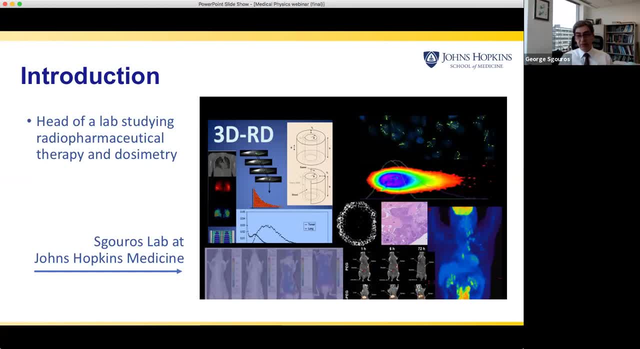 So, kind of, starting from the left part of the panel, you see the 3D ID. Basically that describes patient-specific dosimetry techniques that we've developed in the lab. Moving to the right, you see what looks like a comet. That's the comet assay. 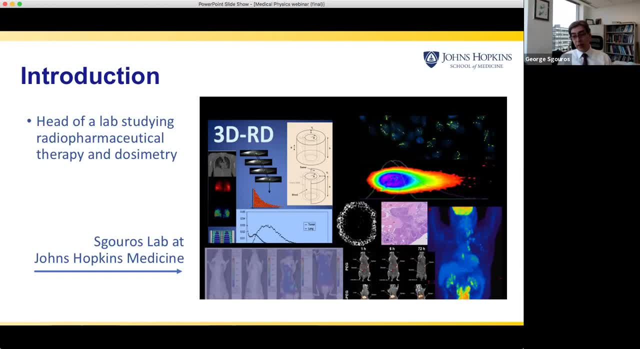 It's used to understand DNA damage and its repair. Right above it you see a bunch of blue-green dots on the blue background. Those are actually alpha particle tracks through the DNA, basically showing how the cell's machinery comes together to repair double-strand breaks. 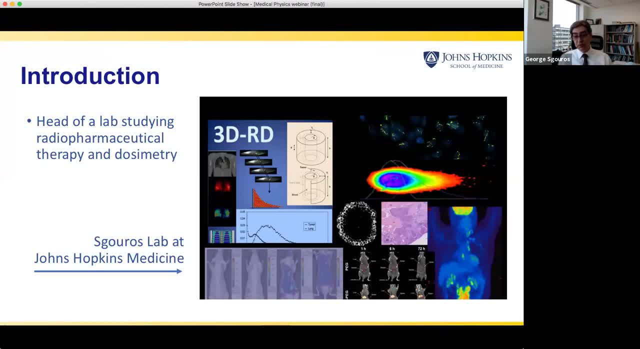 And then below you'll see some mouse pictures. In the lab we do things with mice. And then, above the mice on the right, you see what looks like a sphere. That's an image of a spheroid. It's a confocal microscopy image of a spheroid. 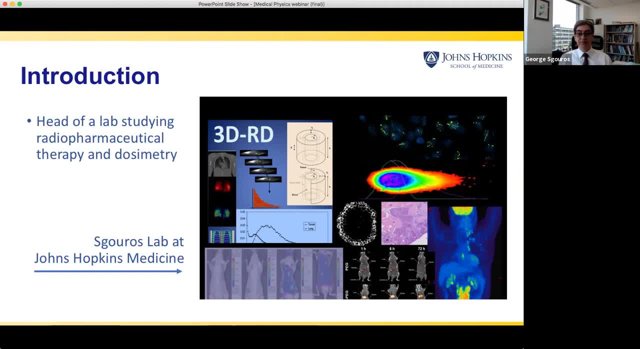 Next to it on the right is a histopathology slide of a mouse. Next to that is an image of an FDG scan of a patient, And in a way, this depicts all of what radiopharmaceutical therapy potentially encompasses, And we'll talk about that a bit more later on. 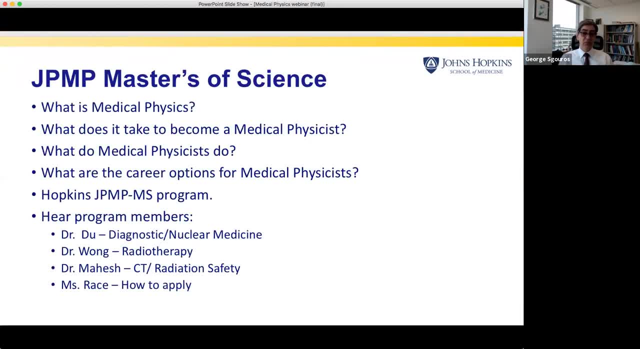 Next slide, please. So some details on the Masters of Science. The objective of this roughly one-hour session is to answer many of these questions, So you'll learn about what medical physics is, what it takes to become one, what they do. 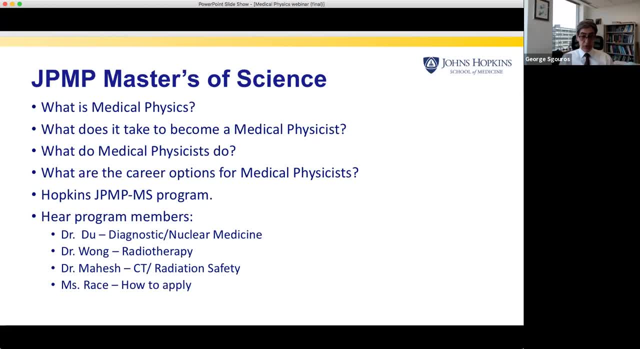 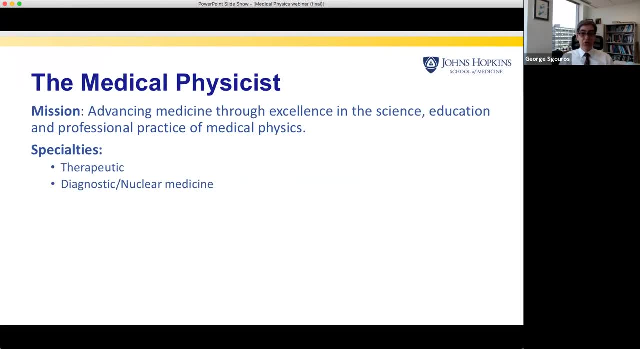 what are the career options and a bit about our program, And then you'll also hear from some of the members of the program Next one. So, starting with the mission statement, it's a very general statement, Advancing medicines for excellence in science, education, professional practice or medical physics. 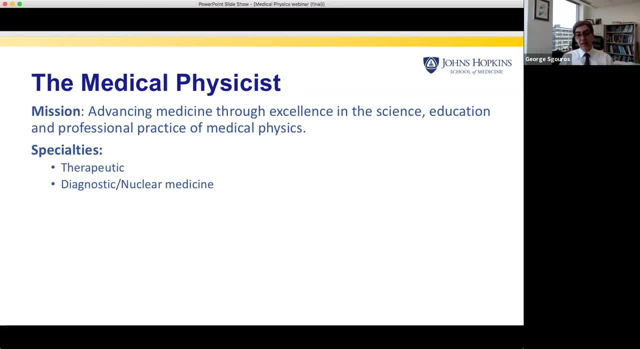 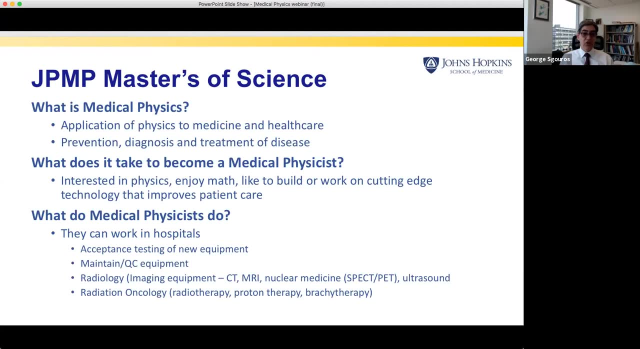 There are two specialties- therapeutic and diagnostic nuclear medicine- And you'll hear more about these later on. Next one. So, moving beyond the mission statement, medical physicists typically apply physics to medicine and healthcare, In particular prevention, diagnosis and treatment of disease. 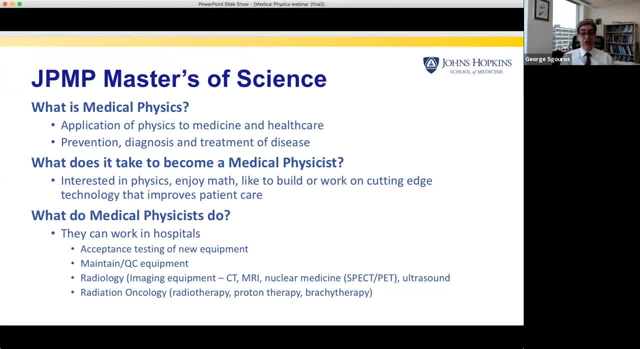 And what does it take to become a medical physicist? So if – and I've encountered lots of people in this situation- They go through high school or undergrad and they like physics, they enjoy math, but they don't really see a pathway forward? 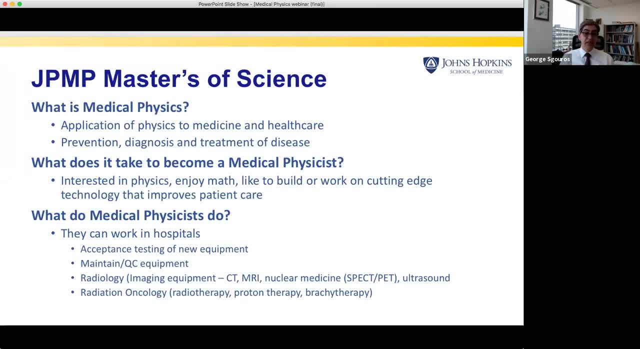 They don't see a pathway to a career. And medical physics is a pathway to a career where you can use the physics and the math and what you've been interested in as you came through your various programs in your education, towards helping patients and applying those physics concepts in a medical setting. 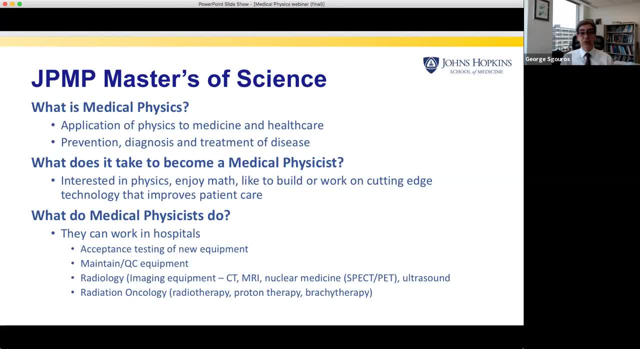 and also potentially working on cutting-edge technology, all of which is intended to improve patient care. So most physical – medical physicists work in hospitals. If, for example, some new piece of equipment arrives, the medical physicist is the first person to take a look at it, evaluate it. 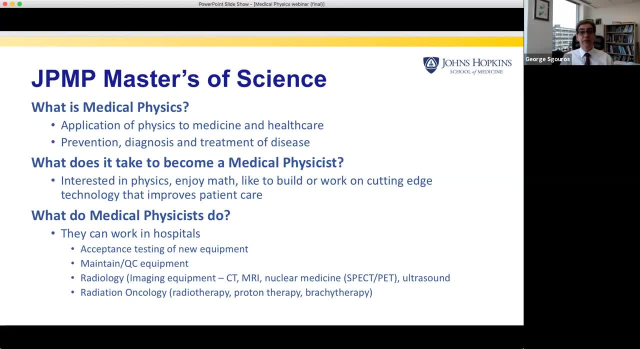 make sure it performs to specs and it's safe to use in actual patient care. Medical physicists in a hospital setting also maintain equipment. They do QC if they're in a radiology that involves CT, MRI, NUCMED, an ultrasound, if they're in a radiation oncology. 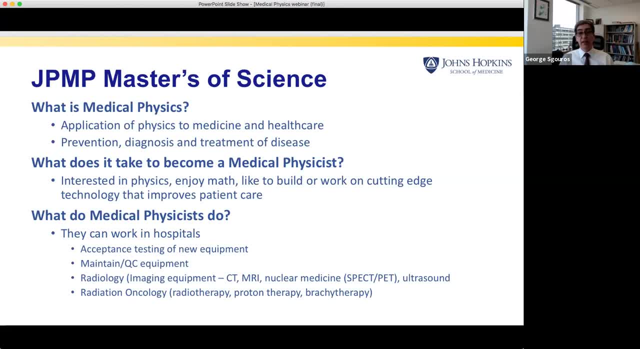 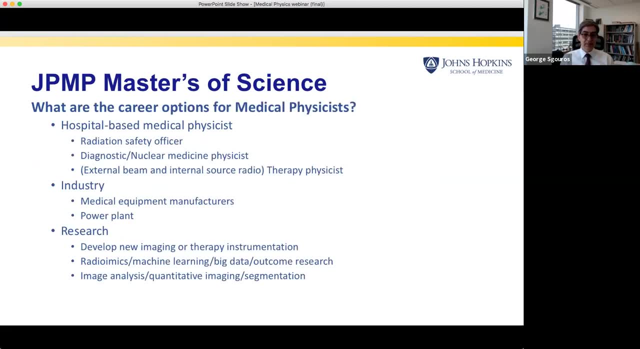 Then it's radiotherapy, brachytherapy and proton therapy, And you'll hear some more details about these in the subsequent presenters. Next, So career options: as I said, hospital-based medical physicists make up the majority Within the hospital setting, radiation safety officers and other potential job opportunities. 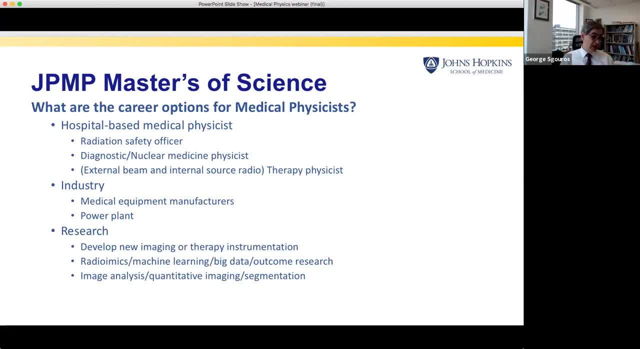 So these jobs are really good jobs. They pay something – starting salaries are around $73,000.. And then depending – for an accredited board-certified medical physicist, And then, depending on career path, they can go up to $200,000, $300,000, and so on. 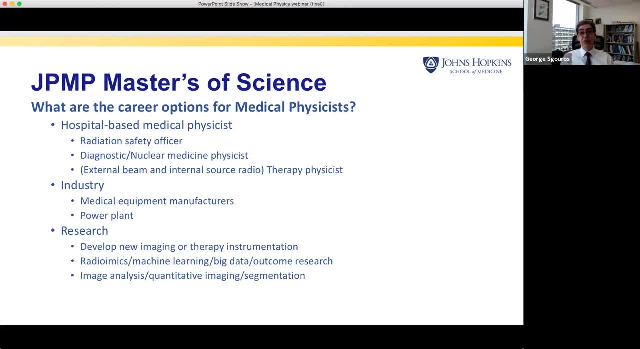 So they're fantastic stable job opportunities And, in terms of a career pathway, they're a wonderful way to maintain your interest in physics and use it to earn a living and develop as an individual on things that interest you. Within industry, there are also opportunities. 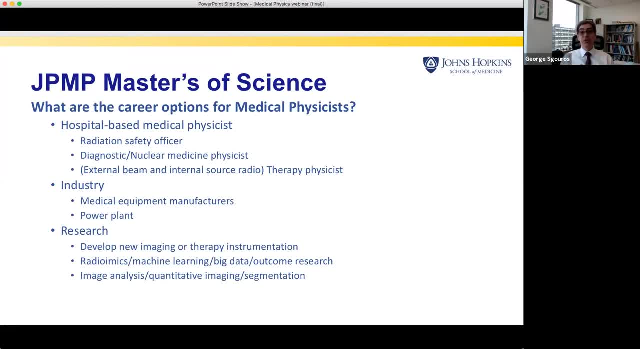 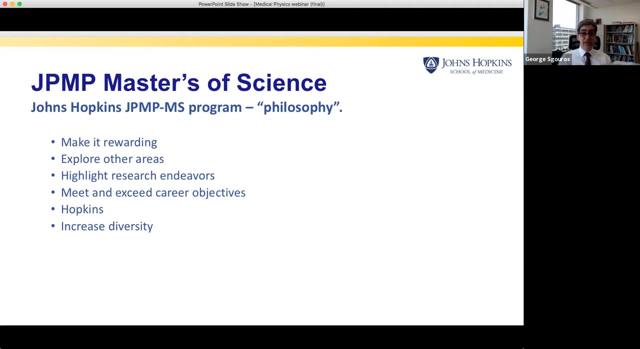 And in research, which is my personal interest. there's a whole bunch of stuff that can be done if you have a physics background and are interested in biology, Next one. So the philosophy of our program first is recognize that this – that we're all keen on doing what's best for the students in the program. 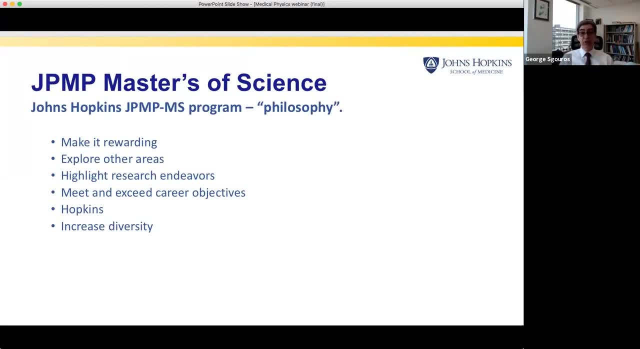 And that kind of amounts to making it rewarding. make your two years as rewarding as possible. We recognize that it's a two-year commitment. We want to make sure that it's as rewarding as possible. Within that context, we want to take that opportunity to let you explore other areas of medical physics. 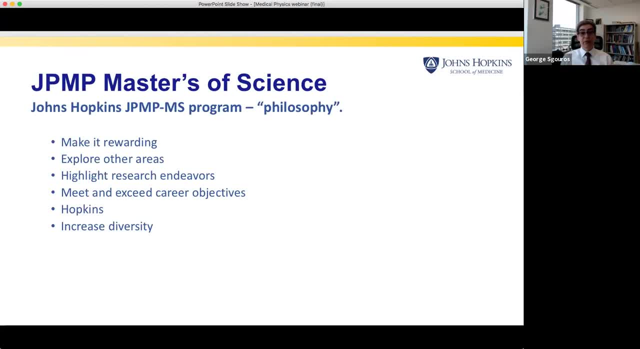 Most people have heard of medical physics in a very specific context, But the point of this program is to expand the opportunities, highlight some other areas that you might not have heard about, to give you a chance to do some research And really to meet – long-term, to meet and exceed whatever career objectives you have. 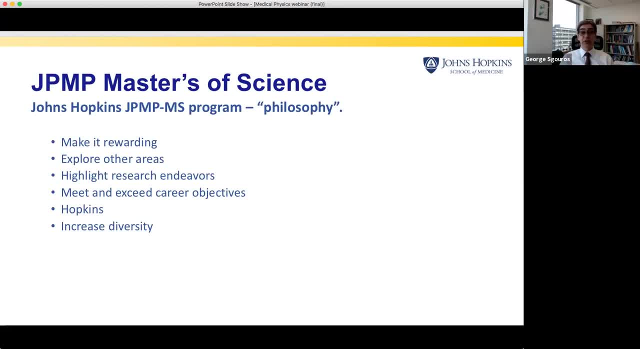 You'll be doing it at Hopkins, which is a world-class, outstanding institution, Amazing research, amazing people And one of the other aspects that I personally am very interested in: medical physics really needs greater diversity, And to the extent we can do this with this program. 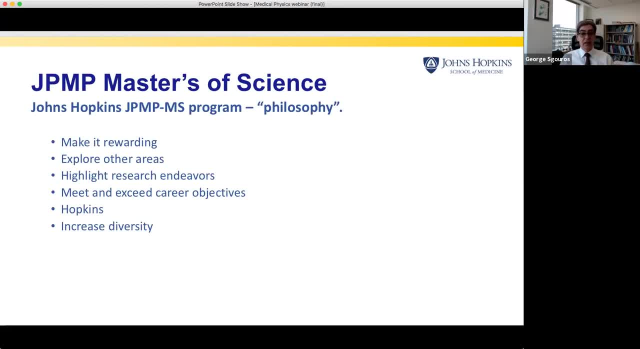 we're going to be looking to try and enhance the diversity, the diversity of voices that go into helping figure out or helping implement medical physics programs in the future. We need mentors and we need – within the field, we need- people that others can look up to and see themselves as medical physicists. 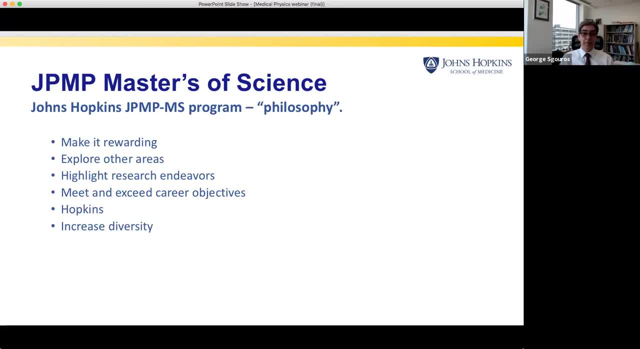 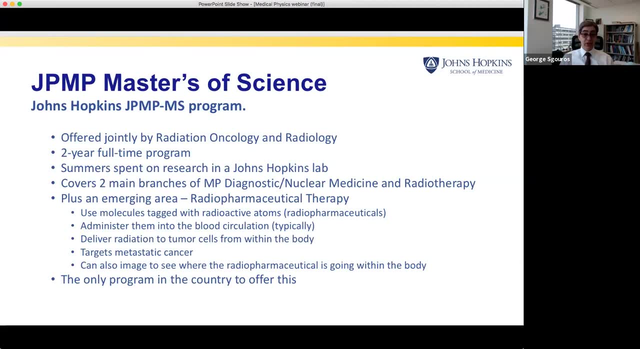 So that's an aspect that I'm particularly keen on. Next, So some of the details. It's jointly offered by Radiation Oncology and Radiology. It's a two-year full-time program. Summers are spent doing research in a Hopkins lab. 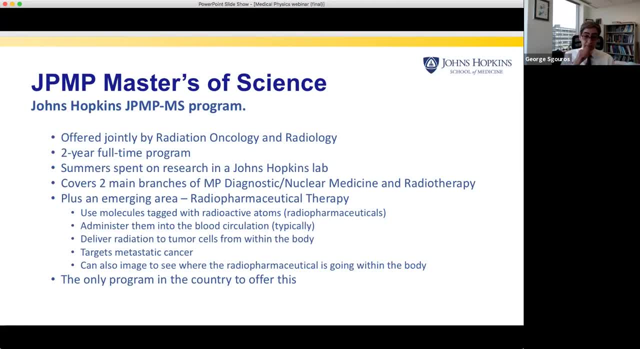 and we have loads of them here, some world-class labs. It's designed to cover both diagnostic and radiotherapy, plus an emerging area which is – you saw that in the initial slide – radiopharmaceutical therapy, which is basically treating cancer cells. 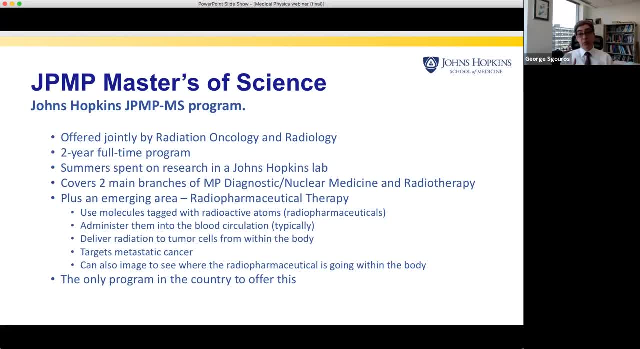 by radiation, where you deliver the radiation from within the patient rather than from outside the patient. The way that's done is you find molecules that recognize tumor cells, tag them with a radioactive atom, administer into the patient. They circulate throughout the body, latch onto tumor cells. 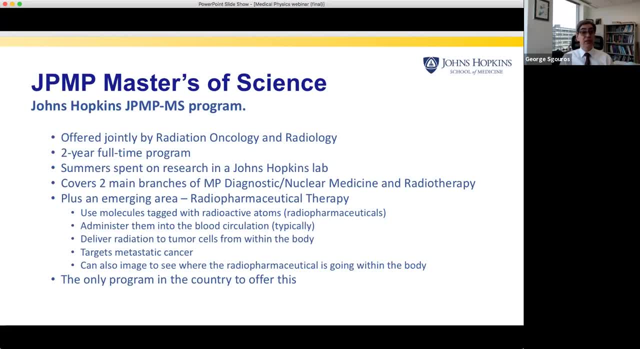 deliver their radiation to the tumor cells. What that means is you can target metastatic cancer, which is really what kills people, with radiation, which is highly effective. The other really important aspect of this is that you can also tag these molecules, and they don't have to be molecules. 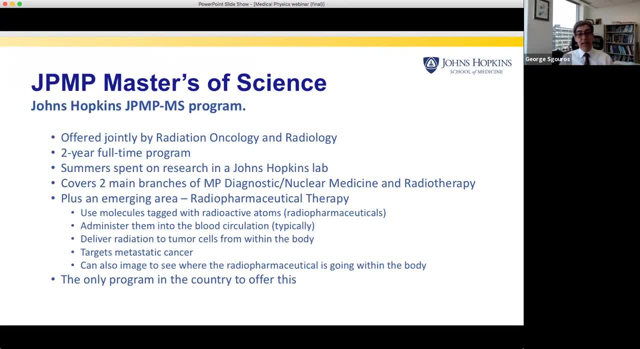 They can be nanoparticles, They can be engineered antibodies, small molecules. You can tag them with radionuclides that also emit photons So you can image the distribution of where they go. You can use those images to do the symmetry to understand the distribution. 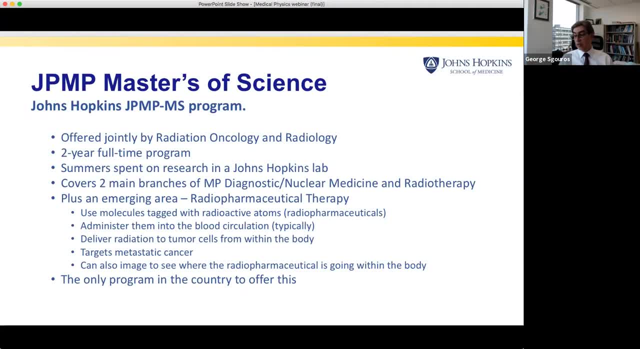 of radioactivity and where the radiation is going, so that you can treat these patients optimally, And I think it's an emerging area. There's a lot of interest from startups and so on, and I think it's the only program in the country to offer this. 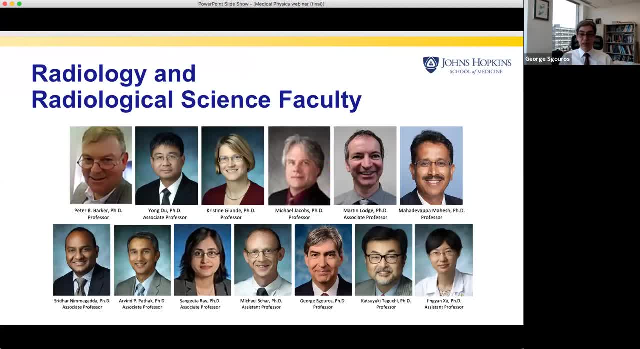 Next one. So this is the group within the program and you'll hear from Dr Du, who is second from the right, and then from the left, And then also Dr Mahesh, who's furthest on the right top row. 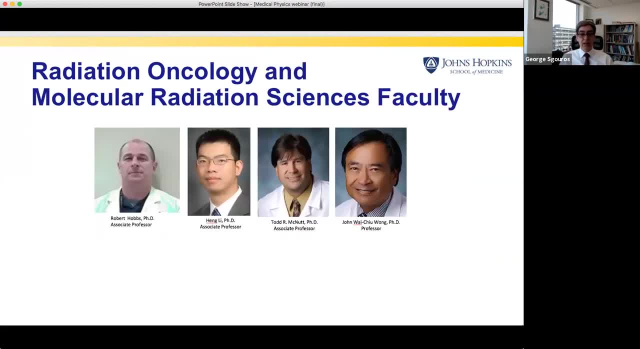 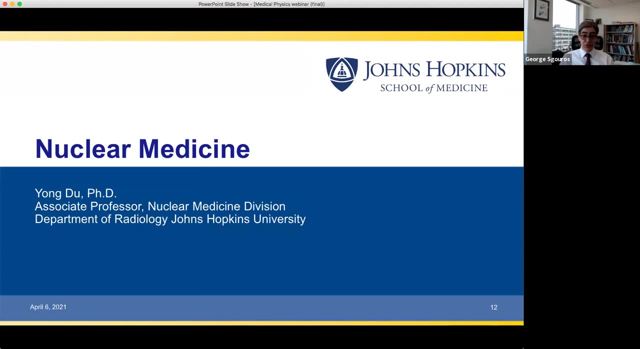 So these are the radiology faculty. Next slide Is a subgroup of the radiation oncology faculty and you'll also hear from Dr Wang, who's furthest to the right. So I now turn it over to Dr Du, who will talk about some of the nuclear medicine aspects of our program. 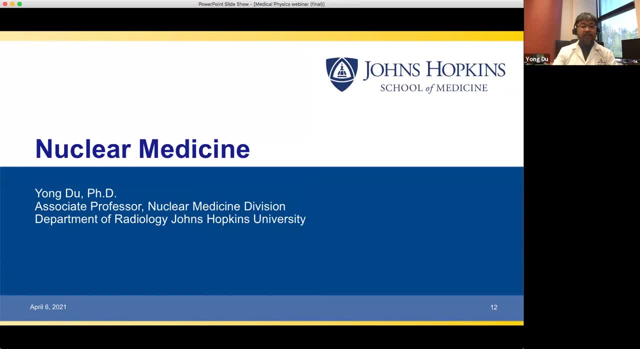 Thank you. Thank you, Dr Garz, for the introduction. Hello everyone, My name is Yang Du. I'm an associate professor in the nuclear medicine division of Department of Radiology. I'm a board-certified nuclear medicine physicist by the American Board of Radiology. 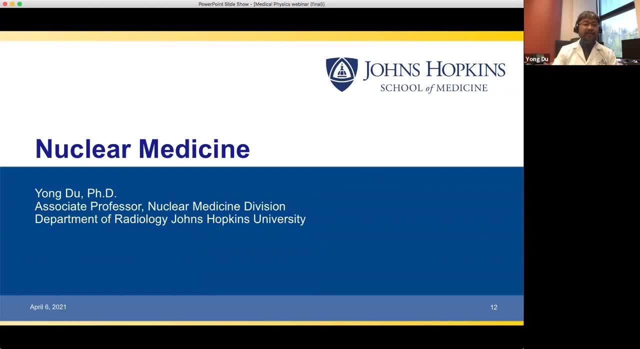 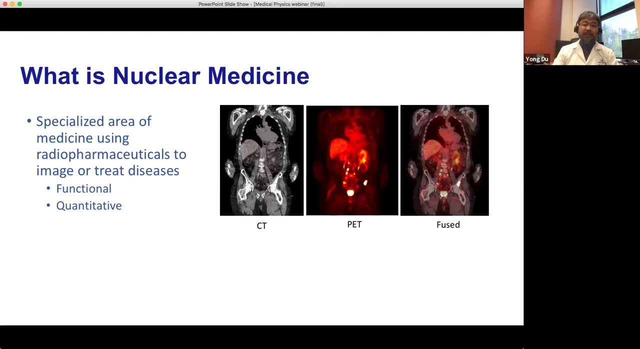 Here I'm going to give you a very simple introduction to nuclear medicine Next, please. So what is nuclear medicine? Nuclear medicine is a specialized area of medicine that uses radioactive material to either imaging or treat cancers, or to do both. So those radioactive material can be a simple chemical compound. 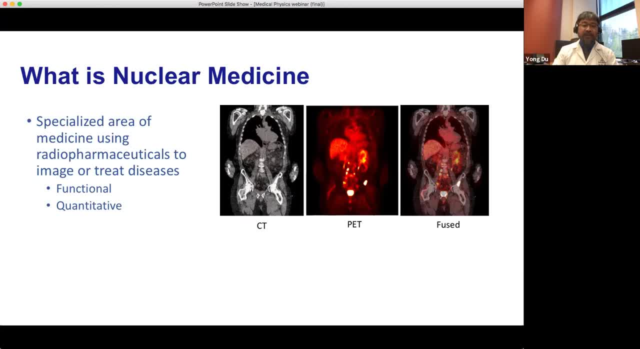 a protein or cells, And they are usually designed to target a specific physiological function. So the nuclear medicine imaging is a representative of the function inside body instead of structures. For example, if you look at the image shown here, the one on the left is a CT image. 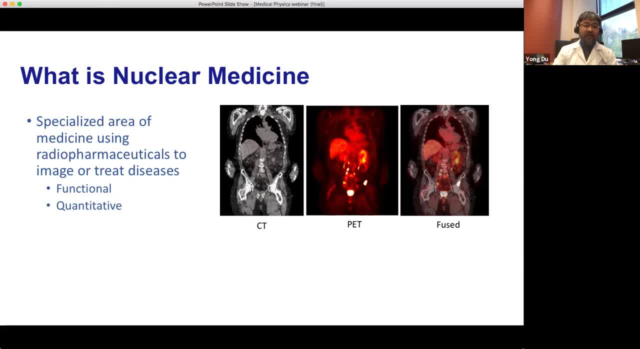 We can clearly see the bones and the liver, lung and other structures of other organs. However, in the middle is the PET imaging. That's a typical nuclear medicine imaging. We can see that those organs are not very clearly defined, But if we look closely we can see there are some very hot spots. 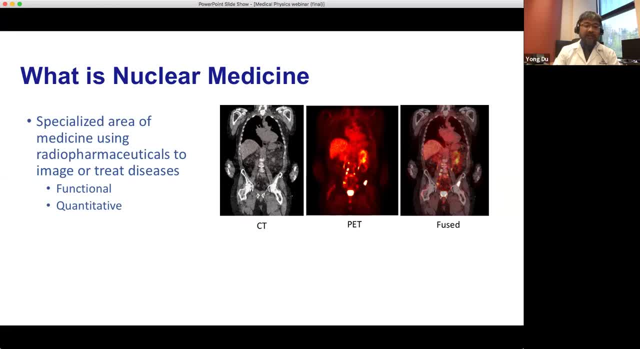 showing up in the pelvic region and in the abdomen. Those are actually the tumors spread from prostate cancer, And usually in nuclear medicine imaging we merge the CT images and also nuclear medicine imaging together to give us an indication of the location of those tumors. 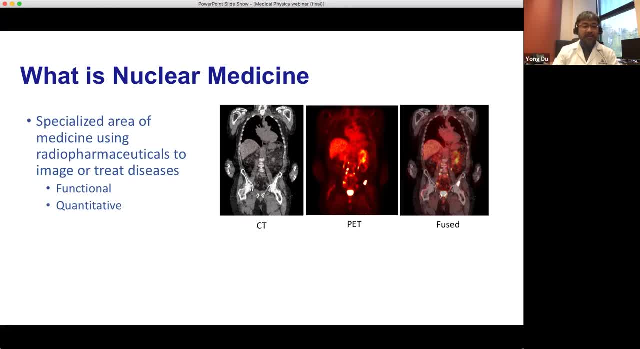 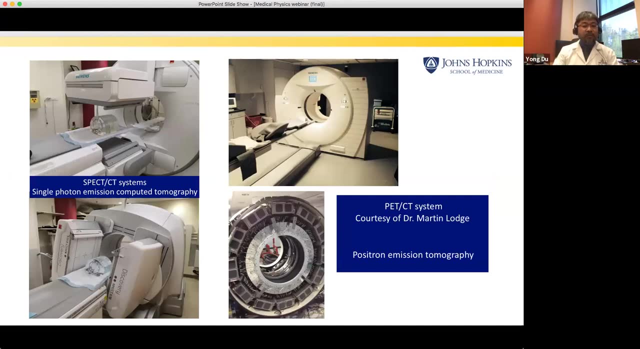 So the nuclear medicine imaging is functional instead of the structure, compared to MRI or CT, And usually we can also measure the uptake in those tumor regions and give us better understanding and classification of the tumor. So it's also quantitative. Next, please. So there's two major equipment used in nuclear medicine imaging. 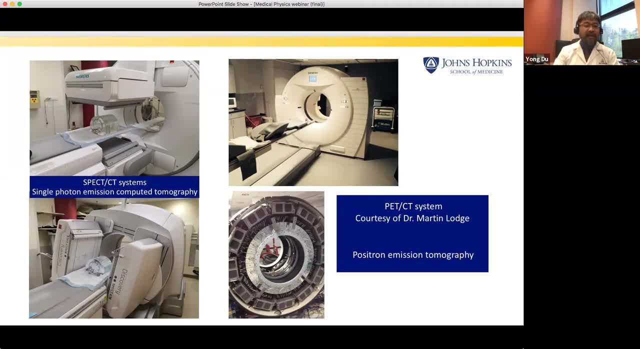 One is the single photon emission computed tomography, as shown in the left. The top one is the Siemens spec camera system and the bottom one is GE, And the other major equipment is the post-tron emission tomography, as shown to the right of the slide. 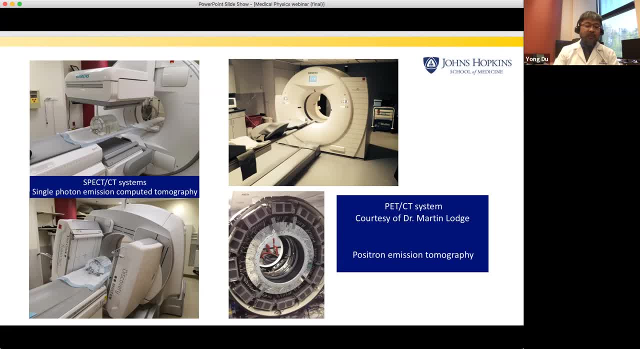 And we can see on the top the Siemens camera and the bottom one is, when they take the cover off, what looks inside. Those equipment are routinely used in the clinic to diagnosis patients and to monitor disease progression and to monitor the efficacy of the therapy. 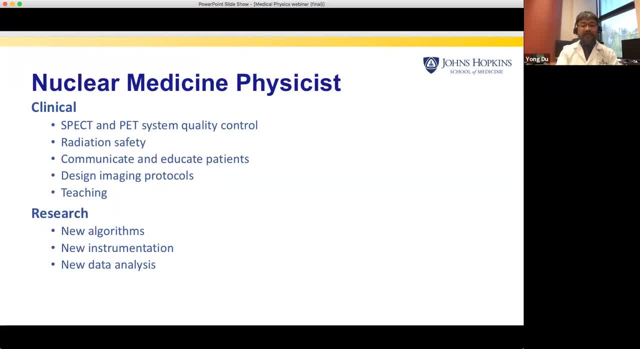 Next, please. So what do nuclear medicine physicists do in the clinic? The major role of nuclear medicine physicists in the clinic is to make sure that spec or path cameras are performing on the highest standard. So this includes performing routine quality controls to make sure the camera is up to the standard. 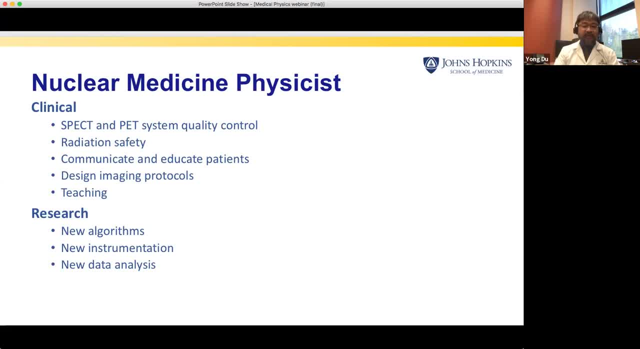 also to prepare the report to obtain the certificate for those cameras. When a new camera comes into the clinic, the physicist's job is to perform testing to make sure those cameras are performed up to the standard. The second job of nuclear medicine physicists is to communicate with the patients. 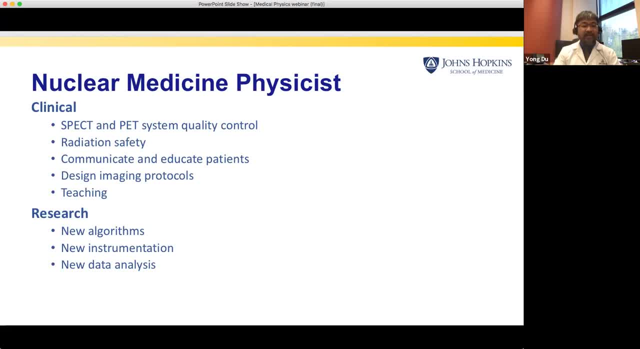 to educate them about rating safety and to address any concerns patients may raise during their treatment or imaging sessions. The physicists are also involved in designing new imaging protocols. When new drugs or new imaging methods develop, the physicist is to implement those in the clinic. 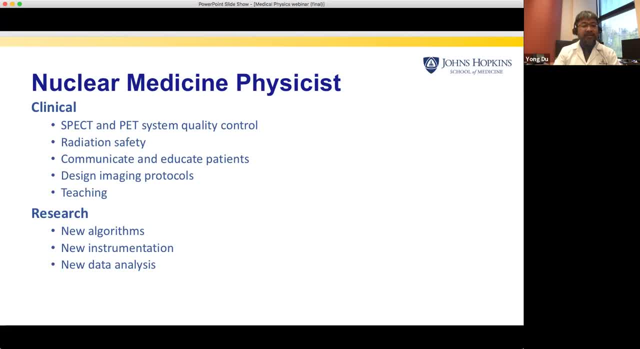 Another major role for the physicists is to teach residents and the interns the basics of medical imaging physics and to help them prepare for their board exams. In the research roles, both in the academia or in the industry, the physicists are usually involved in the development of new algorithms. 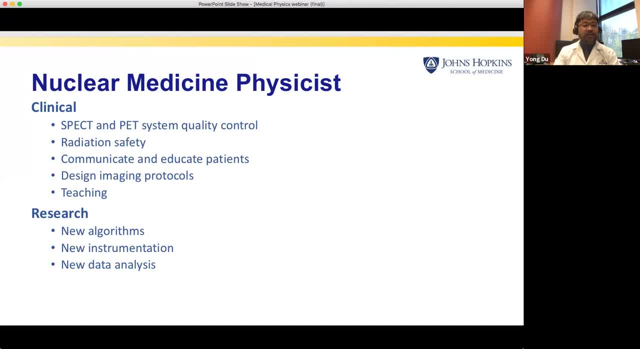 and new methods to analyze imaging and to develop new instrumentation in hardware and new camera systems. They also develop data analysis methods, including AI and big data analysis. Next slide, please. So what will we teach in our program? In our program, we will teach you. 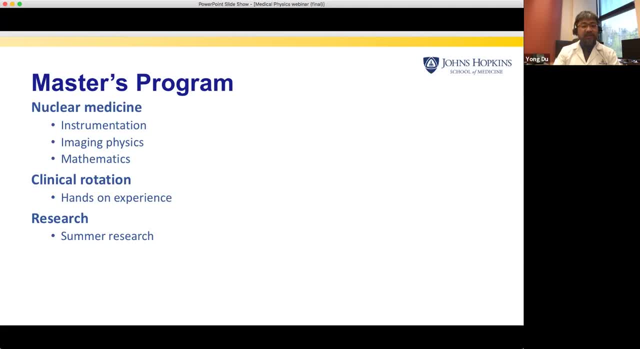 the thorough education of medical physics, including nuclear medicine, including both theory and lab studies. We will teach you the basic physics, mathematics, instrumentation and the clinical aspect of the nuclear medicine. During clinical rotations, you will have a chance to talk with radiologists and technologists. 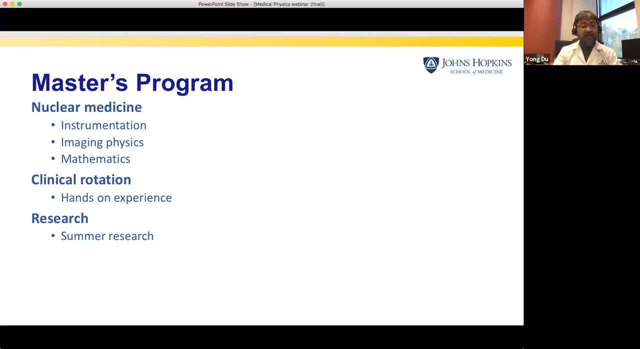 to have an understanding of how the spec and path are used in clinic for diagnosis and treatment, And you will also have a hands-on experience on how to operate those camera systems. In summary, you will also have the opportunity to join our research, to gain first-hand experience. 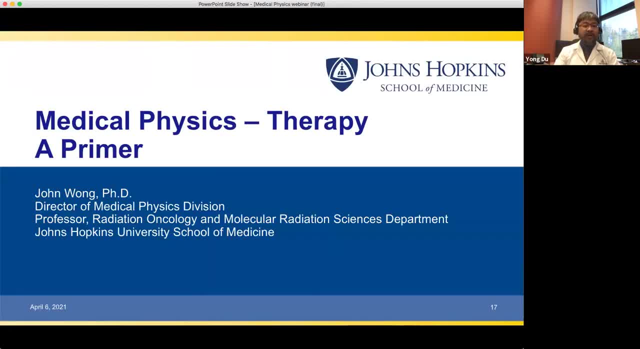 That will be all, Thank you, And next Dr Wang will talk about therapy physics, Thank you. Thank you, Dr Du Hi, can everyone hear me? Okay, Good, So I'm John Wang. I'm the director of medical physics and radiation oncology. 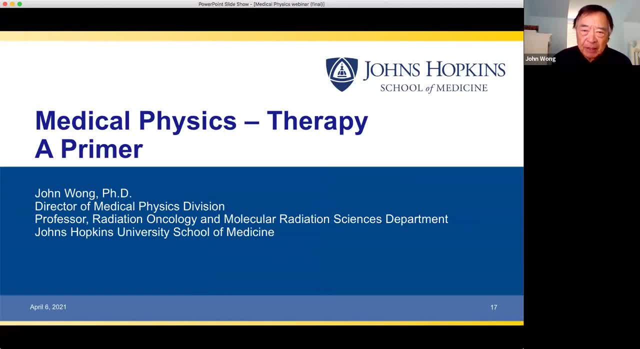 Just a little history. I have been involved in both research, teaching and clinical care. In fact, I spent 12 years of my professional life in the community practice, recognizing this is where the most important part of our profession is to practice good medicine. 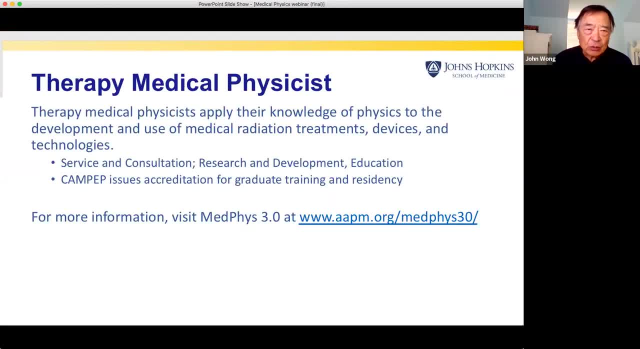 Okay, Next slide, please. Okay. So in therapy, medical physics- we applied our knowledge in the treatment of cancer. mostly, About two-thirds of every cancer patient would have received radiation. So we've become a very large group. We constitute about two-thirds or more. 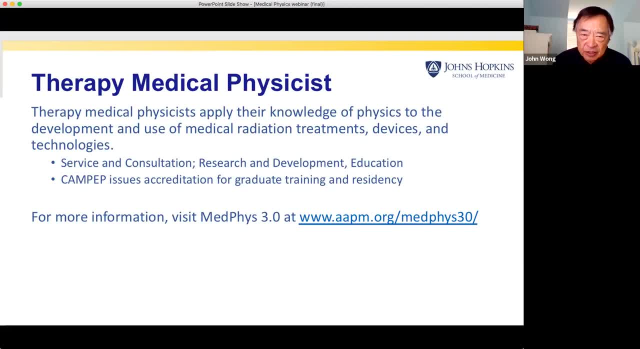 of all the medical physics professionals in this country- And there's 7,000 of us here- We are so involved in taking care of the patient now that we actually have four more in the accreditation organization to make sure that we are professionally qualified to practice. 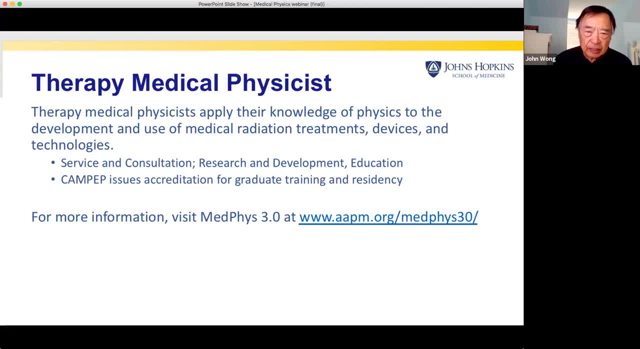 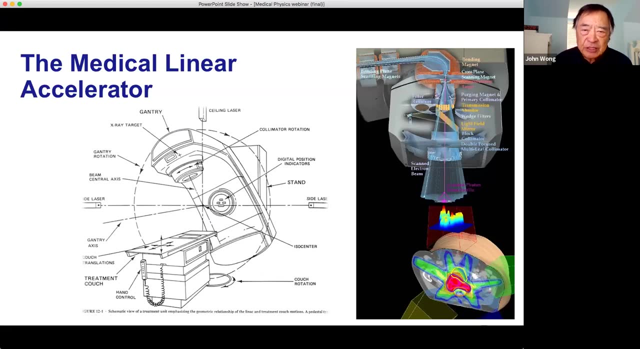 just like the physicians. I think in your brochure you'll be directed to read about what medical physicists do. Okay, Next slide, please. Okay, So just a brief introduction. in therapy physics, This is basically the bread and butter of how we treat patients. 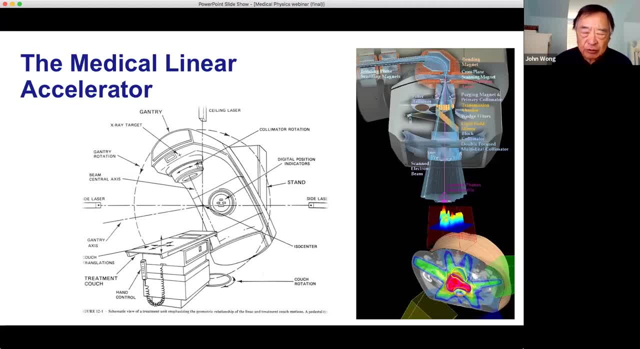 It's a medical. they generate electrons and photons, very high energy electron and photons. Just a description for those of you who, in physics, you know that a light photon is probably about one electron through volt to two electron volt. So we treat patients with X-rays. 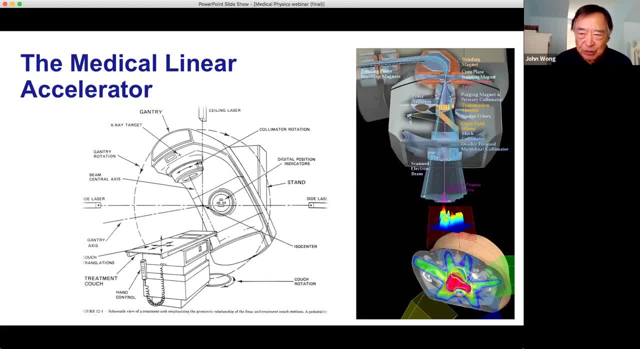 of the order of 18 million electron volt. So these photons are coming through you like particles. So the technology has been around since World War II, beginning in the late 50s and 60s, And that's the picture, the drawing that you saw. 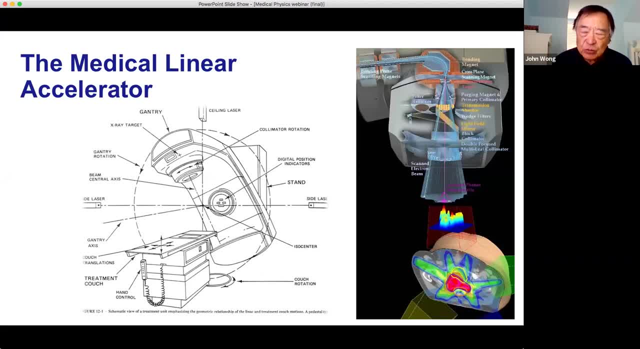 But over the years we have evolved in really good control of the radiation because we want to plan the treatment to a specific site in the patient. It's shown in the bottom right part of the picture that we plan to deliver of the radiation to an atomic description of the patient. 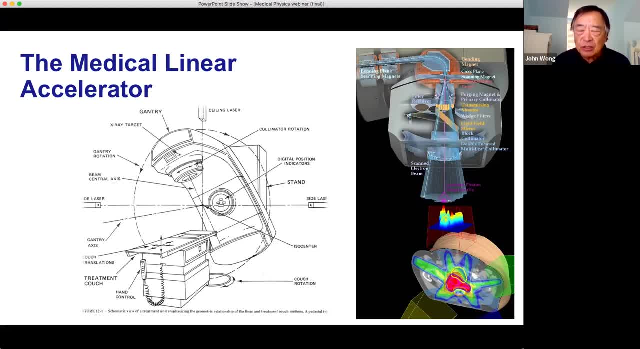 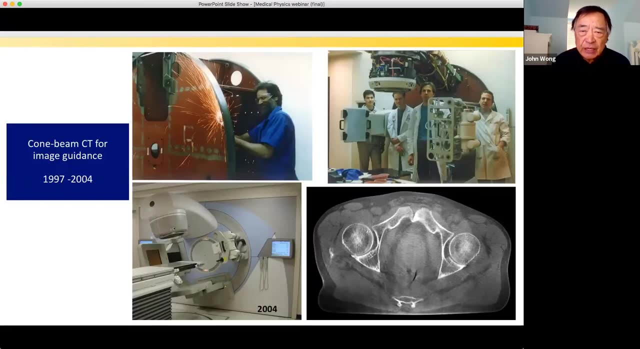 what is MRCT? And then we control the delivery through very, very complex radiation production and modulation of the radiation intensity. Okay, Next slide, please. We actually are very, very involved in driving the field because when we treat patients, we know what is needed. 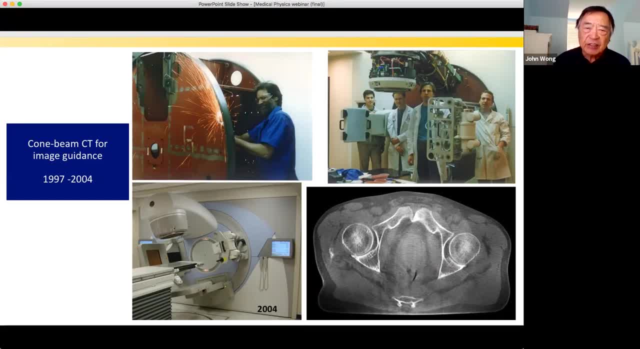 So just a description. Okay, The present standard practice now is called image guidance, And this is actually the fruit of the work by medical physicists that are fortunate to be associated with that. we spent years developing a technique that can actually mount the CT scanner. 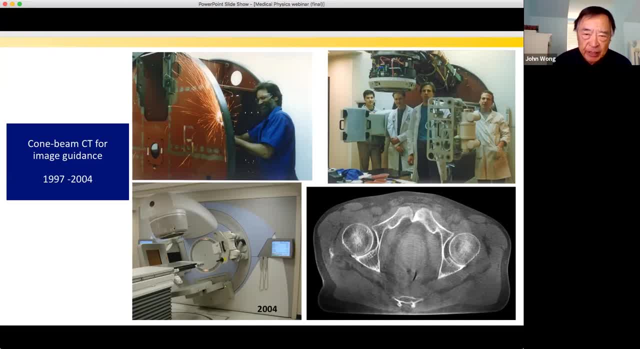 on the medical accelerator. So right now every patient that's come through would have a CT image of them at the time of treatment so they can do better localization or even adaptive treatment to the patient. This is now the standard of care in radiation therapy. 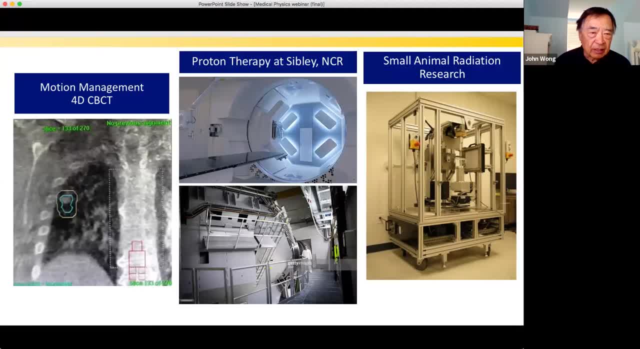 Next slide, please. We do more than that. On the left is actually. it can be a movie, It can be played with, It doesn't matter. We are very much involved in developing motion management, so we actually will be able to make. 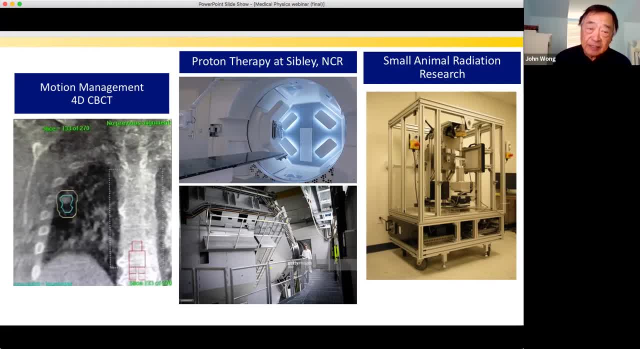 more of these CT images of the patient. This is developed in the field. We now move on to something that we cannot build ourselves, and it's quite extensive. So at Hopkins, now we work. we now have installed a proton therapy center at SIPI in the capitalist region. 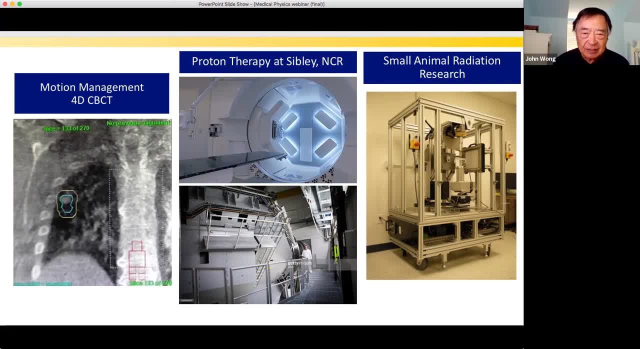 And you can see in the bottom of the middle slides here that this structure is three stories high And you can see one of the physicists standing next to this rotating gantry. Okay, But we also do very exciting things, so we don't forget that we. 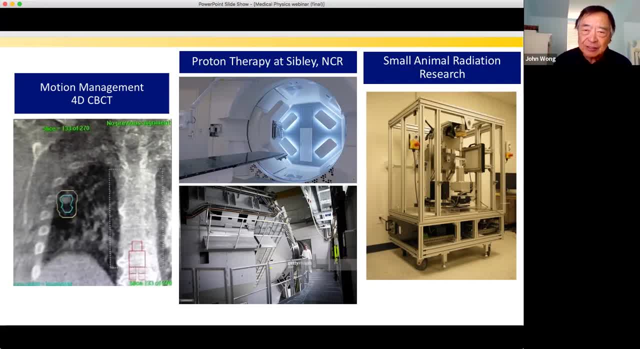 our goal is to treat cancer. We have to recognize that treating cancer cannot be done by one modality alone. So we understand the biology of it. So medical physicists would then have a chance to work with the biologists in the lab. On the right side we show one of the equipment. 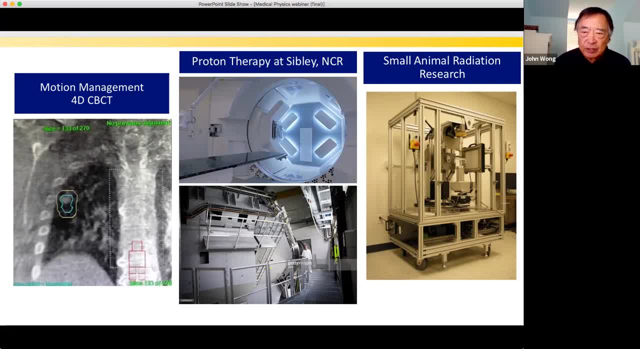 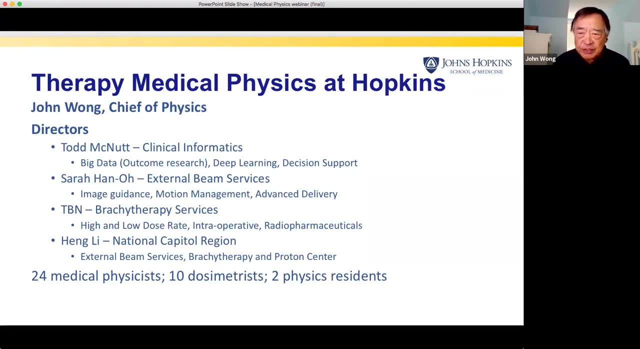 that's being used to treat patients. On the left side we'll show one of the machines that's being used to treat the AI, which is the, has really been the pioneering in the last 10 years- two years at Princeton, So it's a very advanced program. 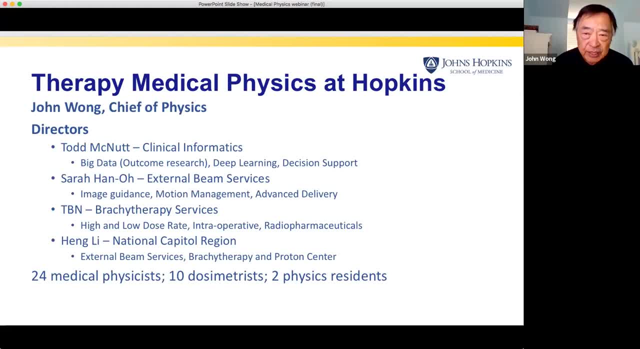 It's a very popular program with a lot of good people, So we will prioritize education and an outreach program. okay, In fact, one of the proudest moments of this program that we have- we're one of the highest funded NIH-funded program in the nation. 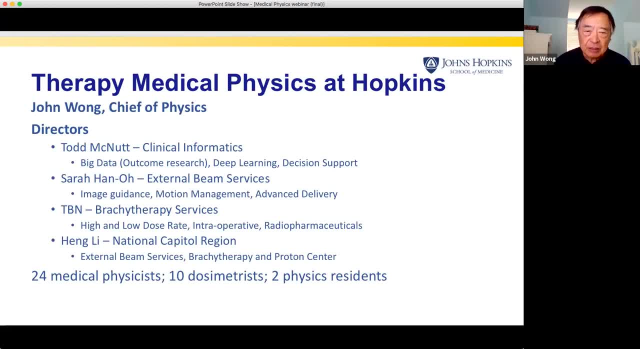 So we want to be able to teach our students good practice, good medicine, and also have a chance for them to look at what's coming. okay, So that's my description of therapeutic physics at Hopkins. I'll pass it on to Dr Mahesh. 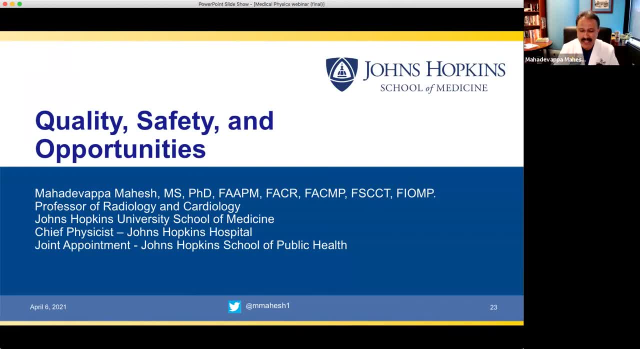 Thank you, Dr Wong. It gives me great pleasure to share some of the things which we are doing and we want to plan to do for the medical physics program. As Dr George Sagouras mentioned, this is a very unique program with faculty involved both in radiology- nuclear medicine and radiation oncology. 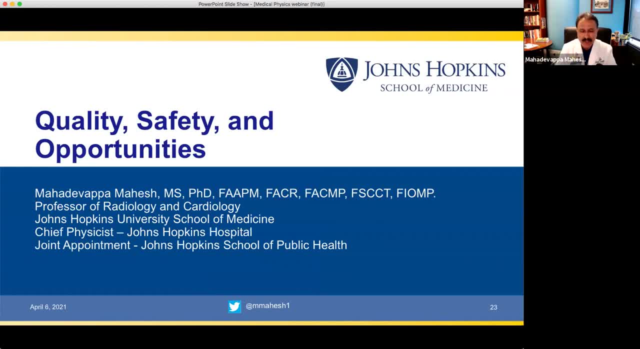 So my area of focus is: I am a board-certified medical physicist in the area of diagnostic imaging physics and I'm also a professor of radiology and cardiology here at Hopkins, And my primary aim is in the clinical medical physics, And I'm going to talk about some of these points. 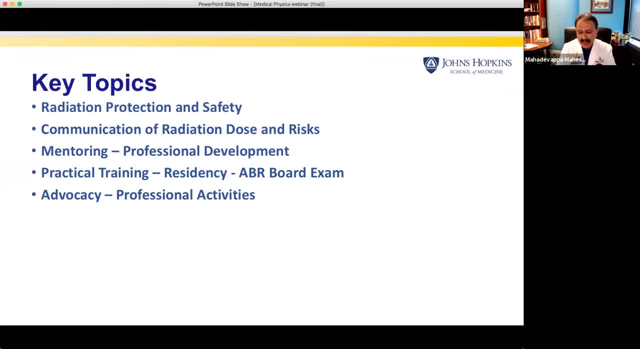 Next slide About things, Because Hopkins gives us a great opportunity, being number one, one of the best hospitals in the world. we have a wide variety of modalities. We have a wide variety of modalities placed in the campus. In addition, most of our faculties are involved in the cutting-edge research. 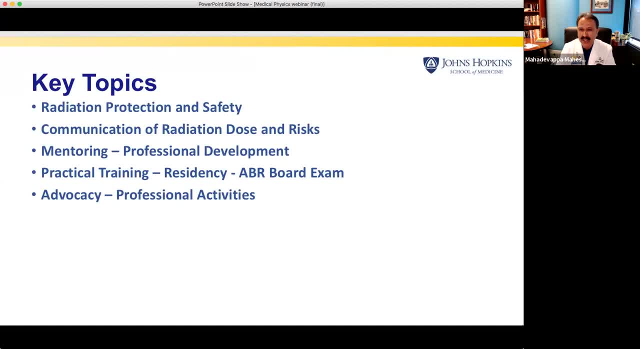 in medical imaging physics and also in radiation so forth. So one of my main focus will be for this program is to teach a core course on radiation protection and safety. As anyone going into medical physics, the radiation protection and safety is very critical. 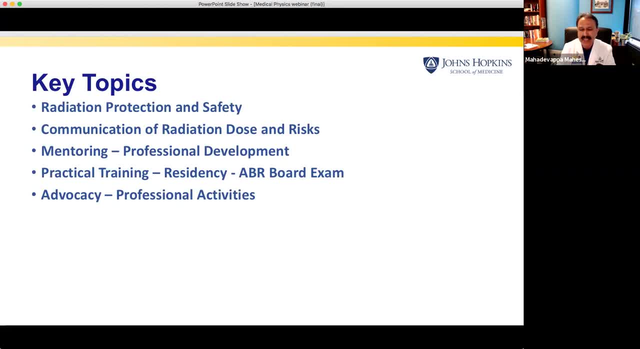 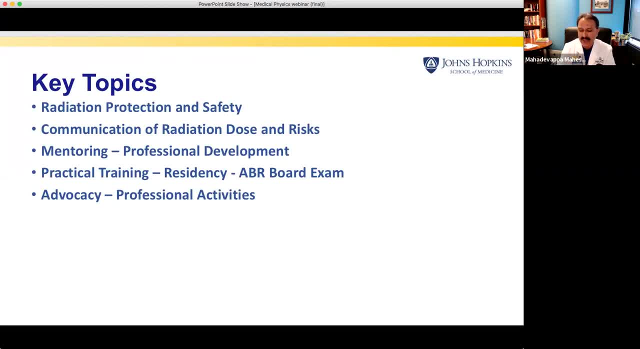 You have to be very careful. You have to be very careful. In addition, radiation protection is very important, not only for self-protection, for surrounding staff protection or patient protection, plus also to be in compliance with regulations. So I'm going to start talking, giving this core course. 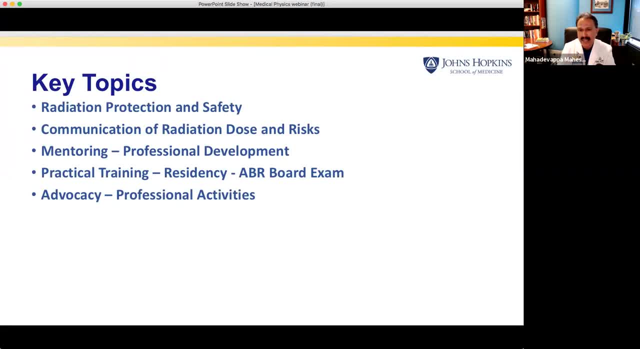 One of the core course for the master's program in the CAMPEP approved master's program is radiation protection and safety and I'm going to be teaching that course to the students. In addition, I'm also very much interested in enhancing the communication capability. 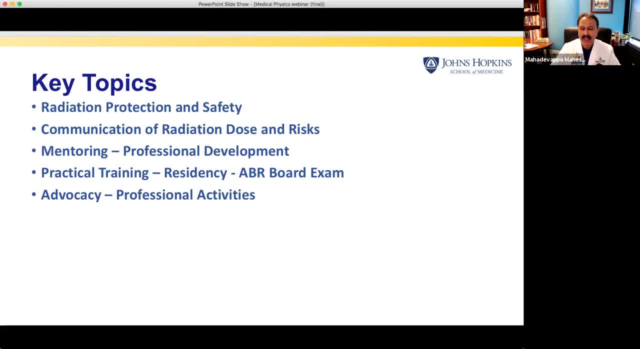 of the students. In addition, I'm also very much interested in enhancing the communication capability of medical physicists, especially how to communicate radiation dose and risk. Anyone working in this field are constantly exposed to these questions about what is the risk for me getting a CT scan. 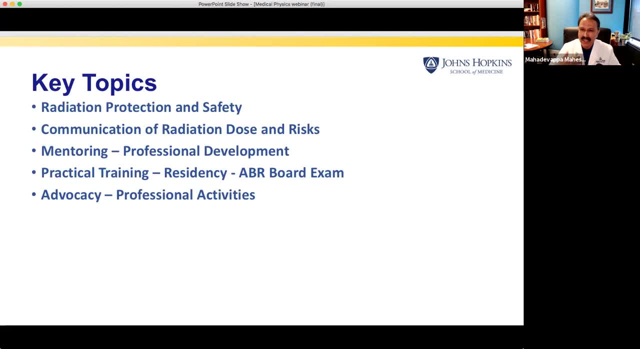 Being in the field of medical physicists, the students, having learned the technology and the physics behind it, should be able to disperse the information or communicate the information very nicely, informatively, to- not only to the users, the patients and everybody, And so I'm pretty much interested in that. 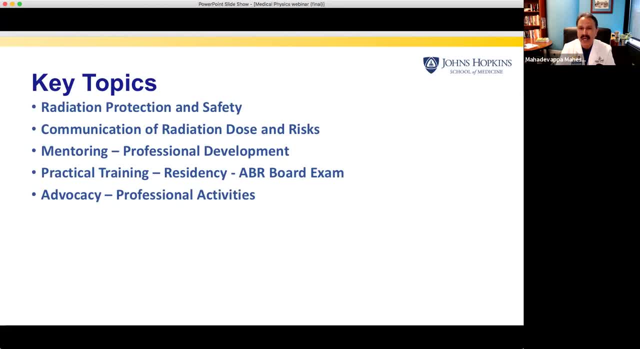 And so I'm pretty much interested in that, And so I'm pretty much interested in that, And so I'm pretty much interested in handling to educate the students in how to learn themselves to communicate the radiation dose and risk information. Also, these days it's very important that, as we are training the students, 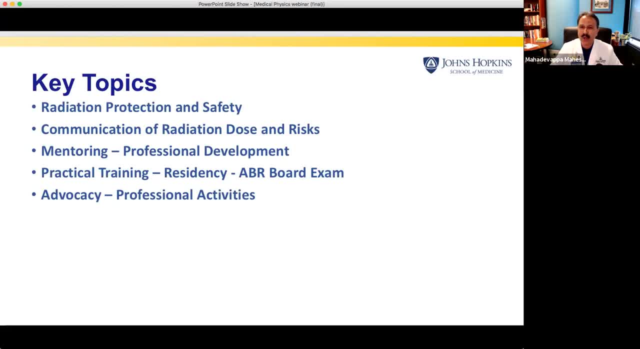 we want to make sure that when they go into profession they are also mentored properly. So that is another area which I'm interested: to provide suitable mentoring to our students, Because we want to prepare our students not just to get a job but also to educate them. And so we want to provide suitable mentoring to our students. So that is another area which I'm interested to: provide suitable mentoring to our students, Because we want to provide suitable mentoring to our students, Because we want to provide suitable mentoring to our students. 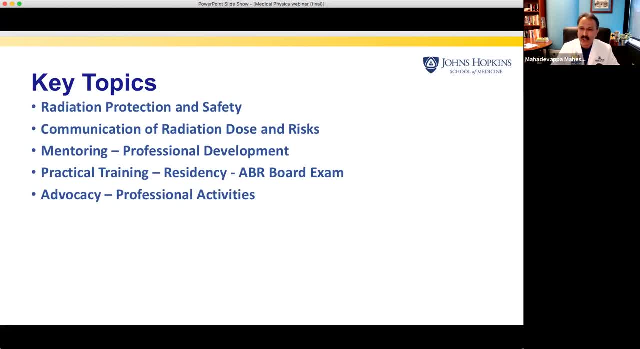 And one way is the students: after the master's program, they can either continue or to do their doctoral studies or they can get into a residency program which will automatically make them eligible to take up the American Board of Radiology Medical Physics, the board exam which will make them. 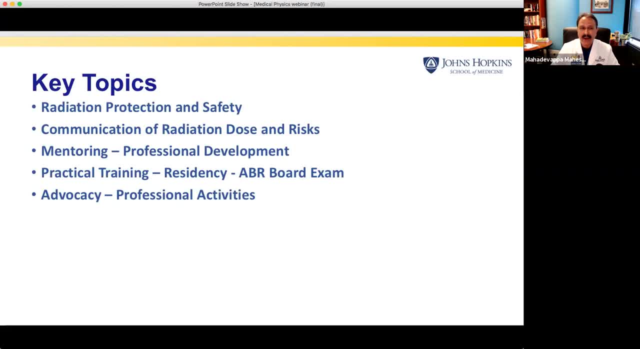 as a qualified medical physicist to practice in the clinic. The other thing is like, as Dr Wong said, majority of the medical physicists- most of them- are based in radiation therapy and about one-third is in diagnostic imaging and nuclear medicine area. 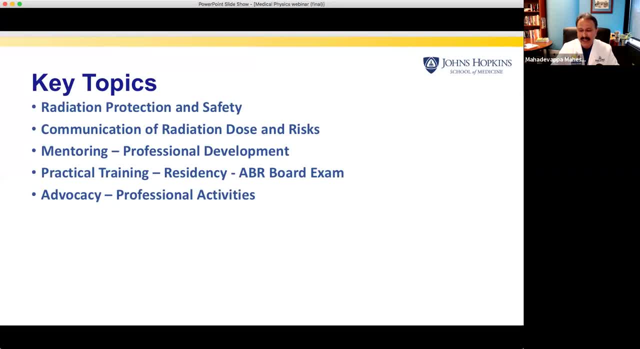 It is also important for us to be part of in healthcare, to advocate our profession in a proper way so that we participate as a good team in catering to our patients. So all these are very important and Hopkins used this as an opportunity because we have exciting faculty working in exciting areas. 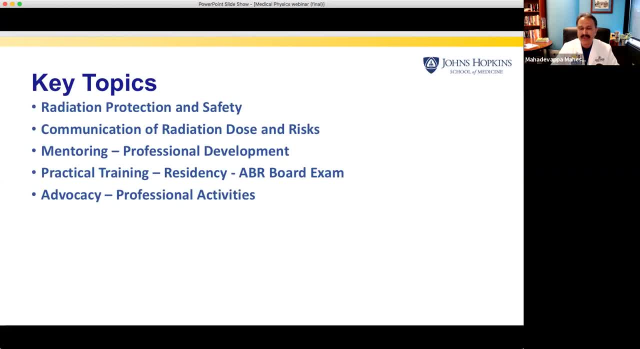 and there's a very nice collaborative atmosphere here. So we want to make sure that we have a good team. So we want to make sure that we have a good team. The students will have the ability to not only study the didactically. 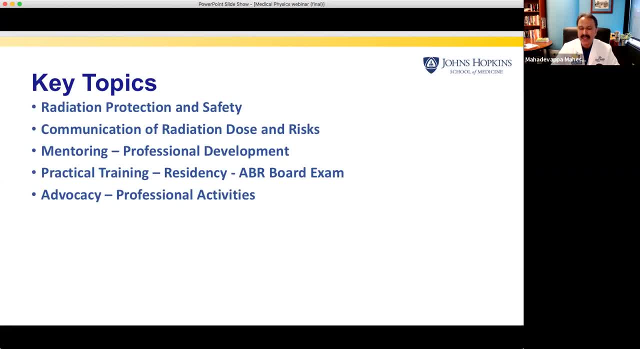 but also learn professionally, not only research, but also regarding the mentor and professional development. So I'm really excited and look forward to this program and I'm giving an opportunity to share our knowledge to the upcoming next stream of students and medical physicists in this field. 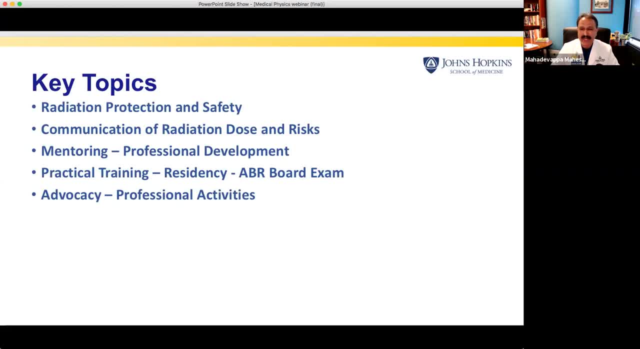 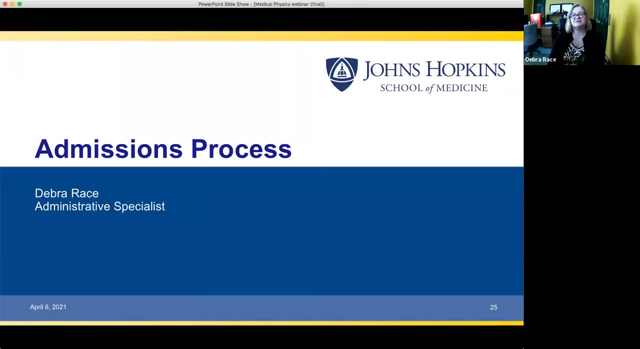 So, having said that, I want to invite our director, Dr Lina Debra Reis, to talk more about the program, Thank you. Thank you, Dr Mahesh. Hi, welcome everyone, It's great to have you here. 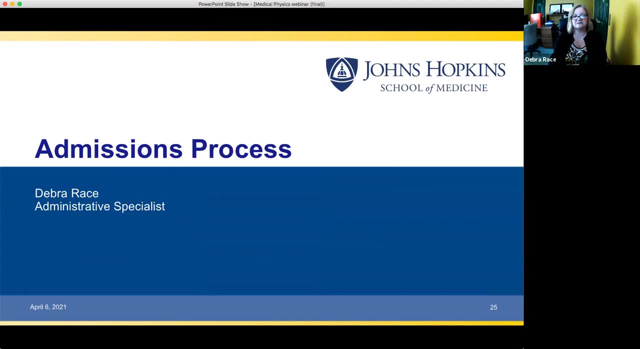 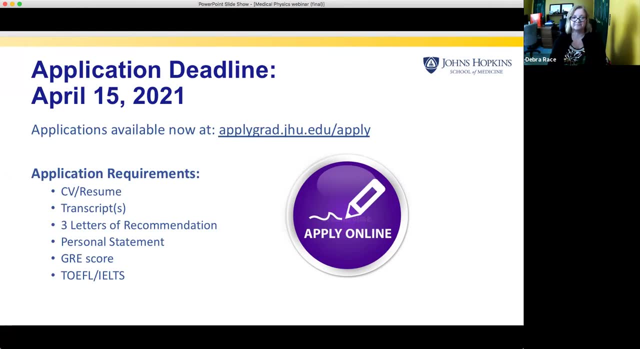 My name is Debbie Reis and I am an administrative specialist in the radiological physics division. I will be your point of contact for prospective graduate students through the complete admissions process. So I'm going to talk to you a little bit about the admissions process here. 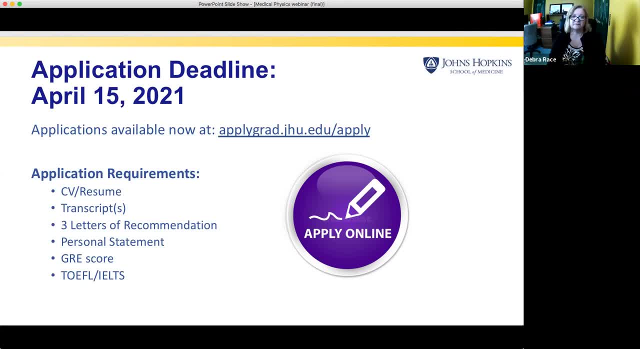 at the Johns Hopkins University School of Medicine To begin the medical physicists. we will only be having admissions beginning in the fall semesters. The process here is a fairly typical one for graduate programs, so it is completely online. The application is now available. 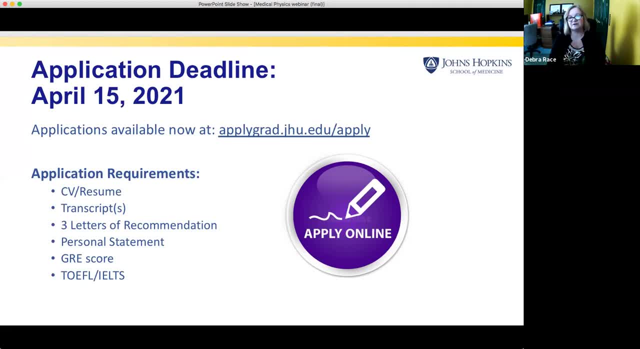 It is linked on our division how to apply page, which we're going to take a look at in a little bit. So these next six things listed are the standard application requirements for our program. These are the main things that you're going to want to have before the deadline. 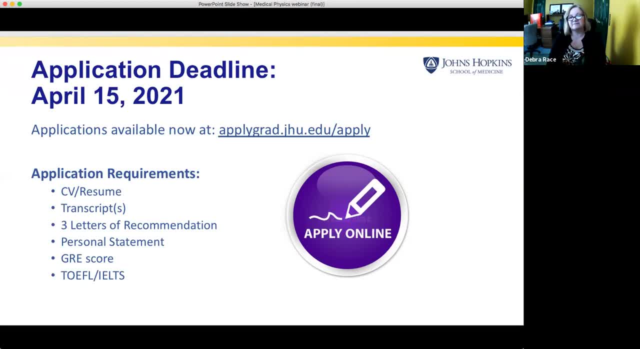 The CV resume is a great snapshot to help us see your educational and professional background. Feel free to include any work experience or research experience with that. Next, if you are applying to the medical physics program, you will have to have an undergraduate degree as well. 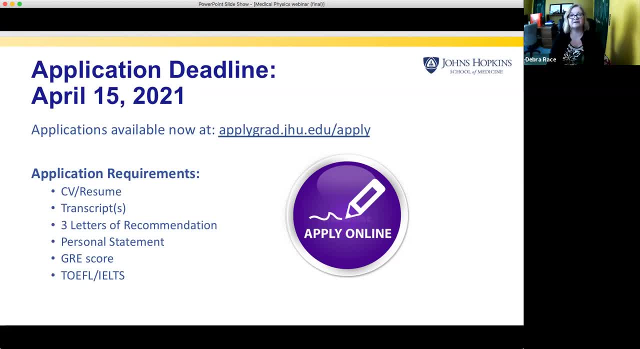 So we are going to need to see transcripts from all the institutions that you have attended or are attending. You will only need to upload unofficial scanned transcripts or electronic transcripts For the review process. another really important part of our application is going to be your letters of recommendation. 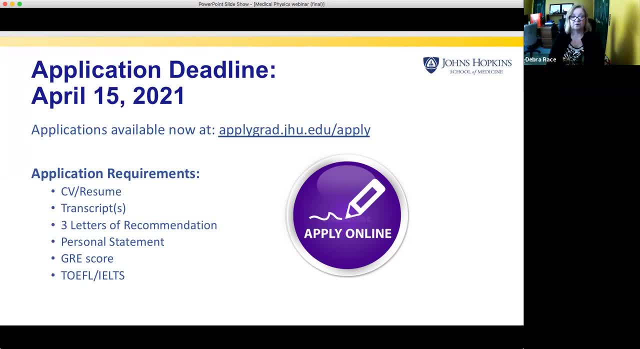 We do require three letters submitted with your application. What your recommenders get to do for you is to really help us understand in another way what your capabilities are. I've often been asked about who should write the letters. You want to have people who know you well enough that can vouch for your ability. 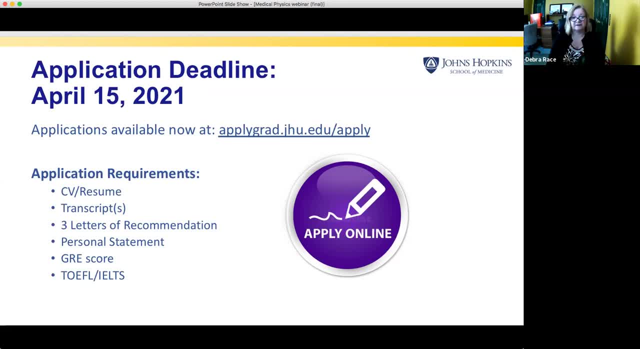 to do well in a graduate program And most of the time, these recommenders are going to be your academic professors. What's most important is that your recommenders have personal knowledge of your abilities. Next, in the personal statement, we want you to focus on what attracted you to our program. 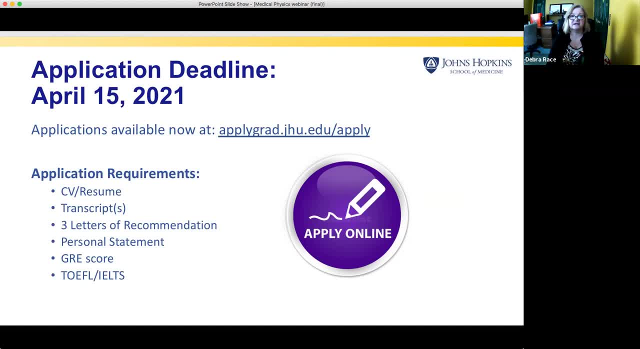 what is your short and long-term professional goals? and then a little bit about how you prepared yourself to be successful in a graduate program. I always encourage applicants to think of this as an opportunity to learn more about yourself, and that you have the opportunity to share your story. 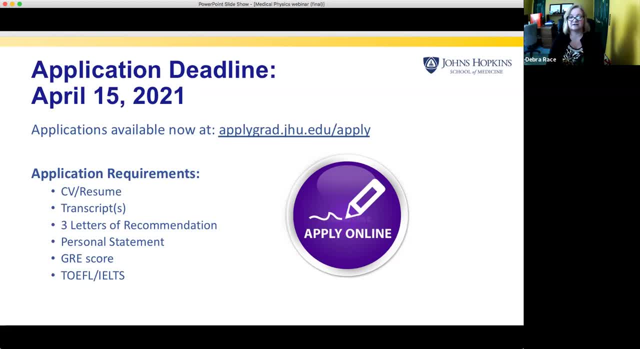 Another thing that I encourage applicants to consider talking about in their statement is if you have any concerns about your application. So, for instance, if you performed poorly during a semester and you want to explain what happened in that semester, we'll include that. 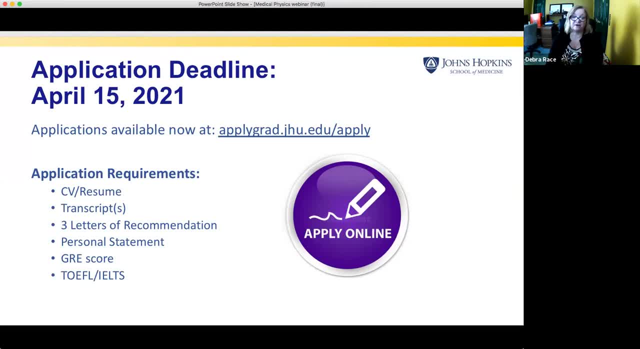 We will see all elements of your application. So if there is a red flag on your transcript or somewhere else in your history, we suggest addressing that rather than leaving it as a question mark for us. We do require the general GRE exam score. 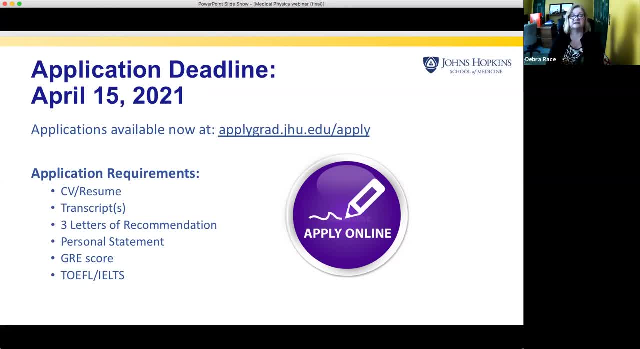 The physics GRE is not required, but it is recommended. Caveat to this is due to the COVID-19 pandemic. the division is going to waive the GRE requirements for the fall 2021 admissions only And if you are an international student and you studied outside of the US. 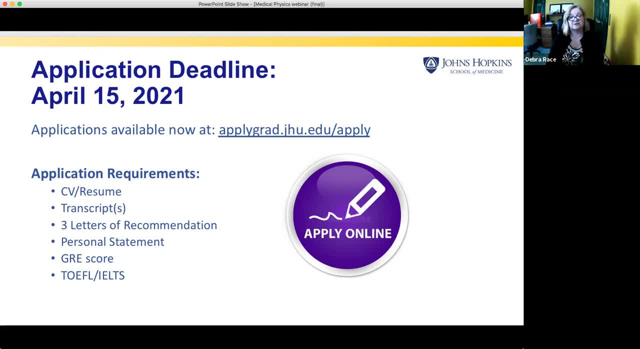 for your undergrad in a country where English is not the official language, then you will need to take either the TOEFL or the IELTS test to show evidence of English as a second language for the English language proficiency. Next slide, please. 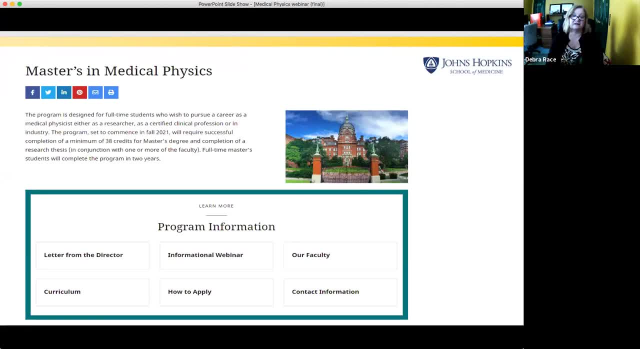 So here are several of the most useful pages, webpages that you'll want to visit. The first page is from our division website, which can be easily found by Googling radiological physics division, and we pop up right there at the top. 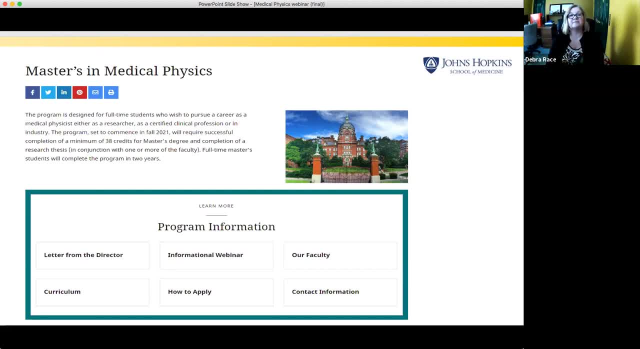 This is where you can learn more about the master's in medical physics program. You can see a wonderful introduction by our director, Dr Chigouros. You can learn about our curriculum, our faculty and, most importantly, how to apply. 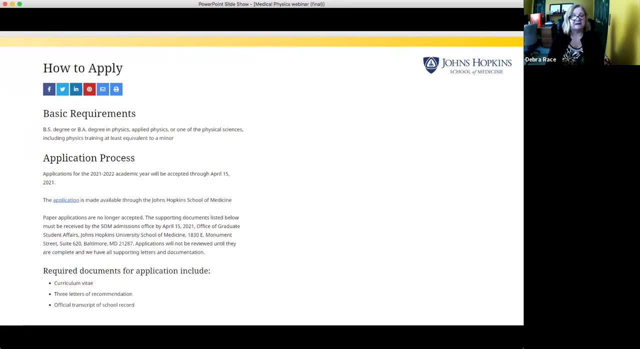 Next slide. So the next page will give you more information on how to apply, and this is where you will find the link to the online application. This will take you to the Johns Hopkins School of Medicine on-campus graduate programs, with the date that the application is available and the deadline. 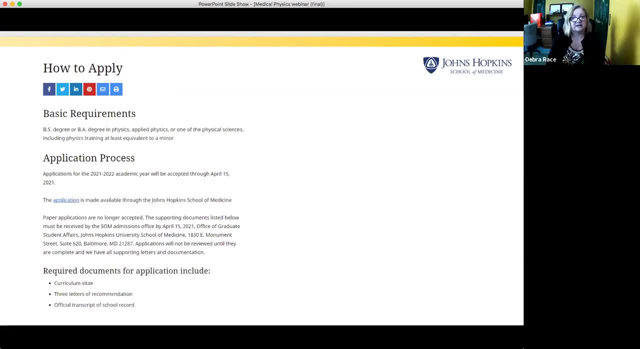 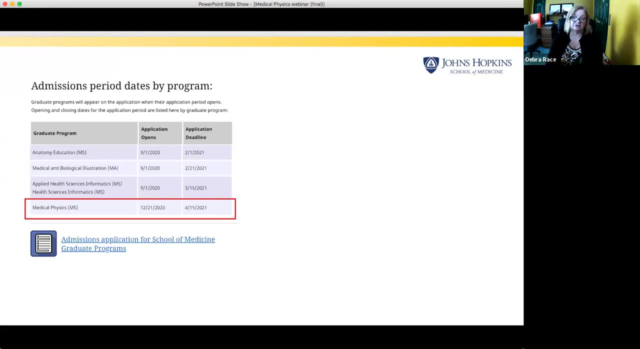 Below medical physics. there you'll find the admissions application. So once you select that next slide, please. you will land on the graduate admissions page. You will create an online account. You can move through the application at your leisure, saving your work and returning as needed. 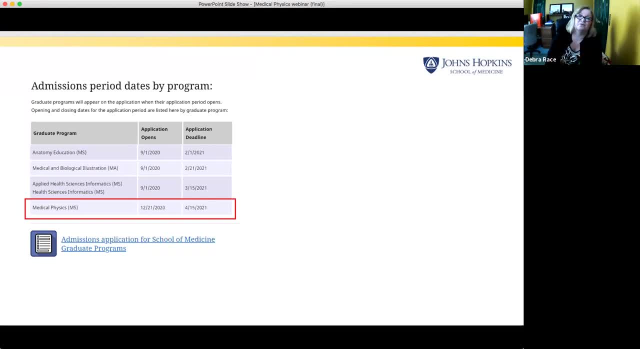 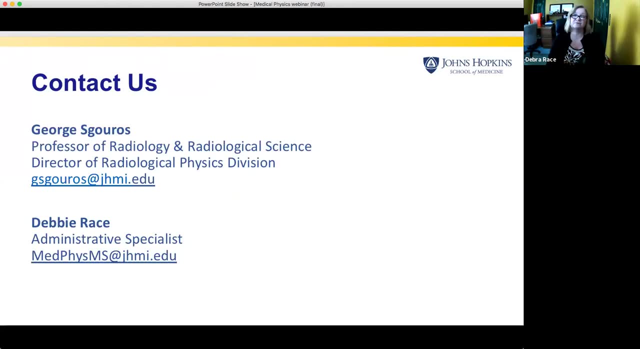 I hope this information was helpful to you. I thank you all for being here with us today. If you have any questions, please contact us at any time. We would love to see your graduate applications and, with the hope that we can actually have you join us in the future, 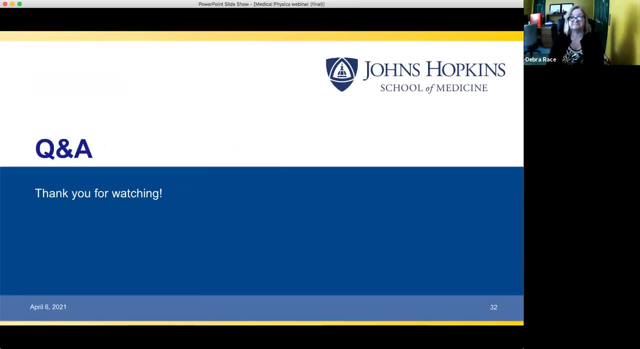 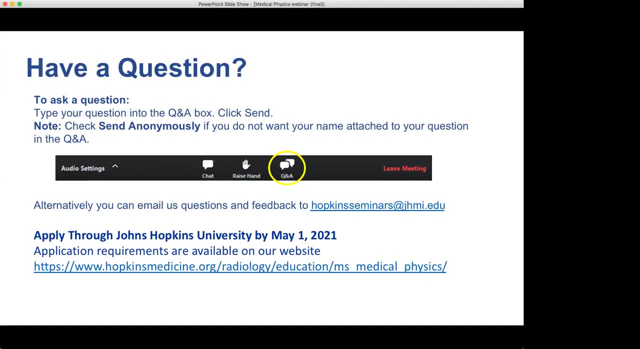 So now we will start with the question and answer session. Okay, it looks like we have a few questions already submitted. The first question is: we have a student interested in the program but would like to learn more about the that is offered. 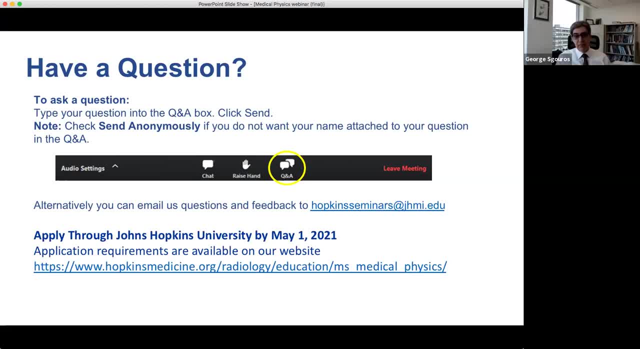 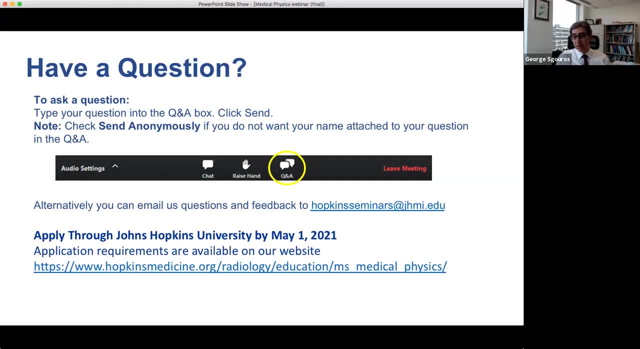 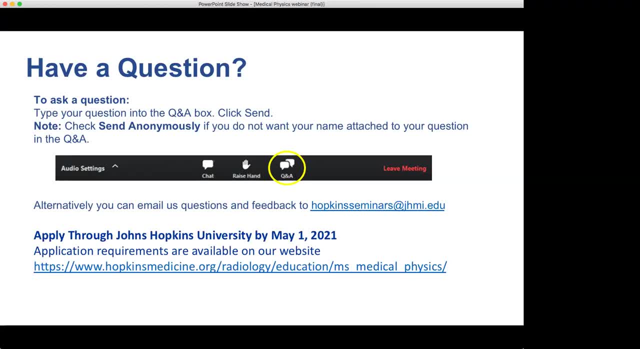 about the financial assistance or financial aid that is available. So, Debbie, I think you're probably the best person on the panel to answer that question. Debbie, you're muted, Sorry. Yes, So we do have a great financial aid office here at Hopkins. 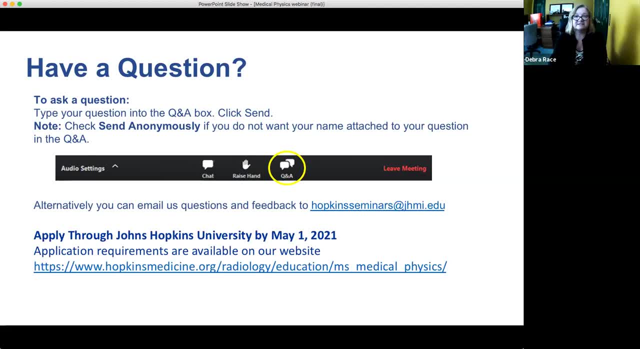 that can answer a lot of these questions. So, since this is just a master's program, there is no financial support within the program, but there are avenues for students to apply for federal direct loans or other graduate type of loans. So we always point applicants and students into the direction of the financial aid office. 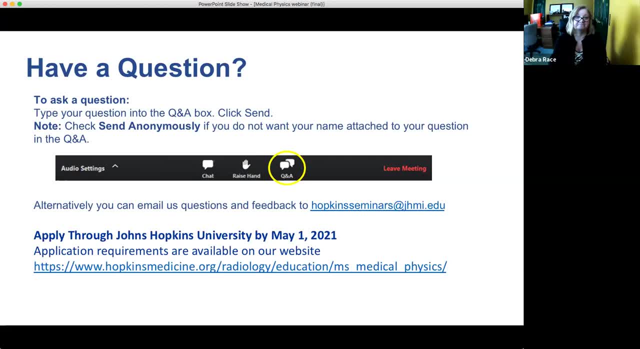 Great. Another question is: what is the best way to apply for federal direct loans? So the question we have is: what classes do you recommend students take in undergrad to prepare for this program? I don't know that. we have a specific set of requirements. 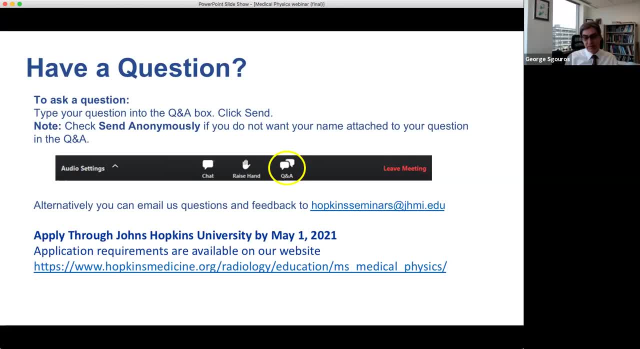 Certainly physics and math would be important and sort of the higher the level, I think, the better for this area. Mahesh, or Jan or John, do you want to elaborate? Yes, I can just tell you the background of people that went to therapy. medical physics includes all types. 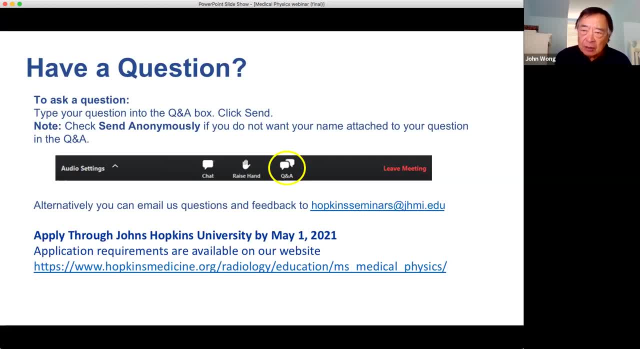 of engineers- electrical, mechanical, computer science folks- okay, and also general physics. Usually you should be good at math and computer programming, Like I would recommend students be able to do different things. Like I would recommend students be able to do differential, partial, differential equations okay. 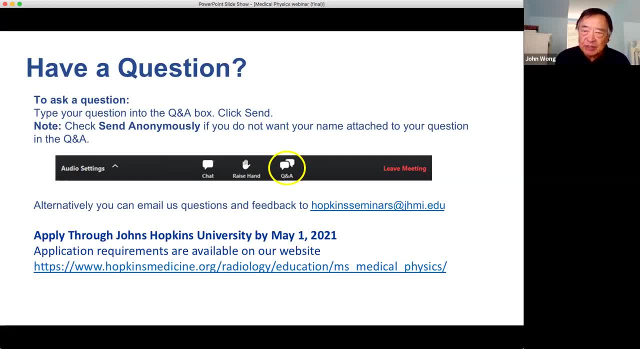 That was not a prerequisite, but it's desirable- and some knowledge of the core physics, like electromagnetic wave theory, nuclear physics and the core courses. Does that answer your question? Okay, Mahesh, do you want to add on to that? 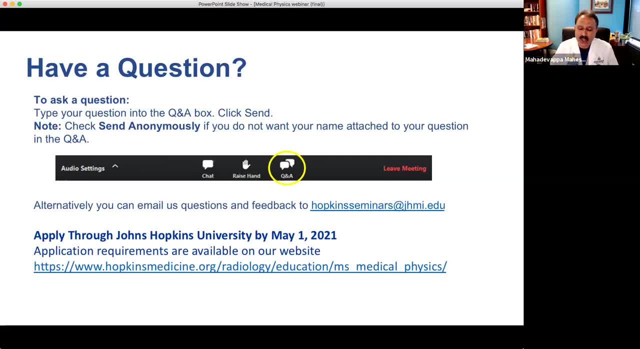 Yeah, I think a solid applicant. It will have a strong science and math background. Not necessarily like a particular course, but need to have good and also, for example, in the higher level in the fourth year probably should have an exposure. 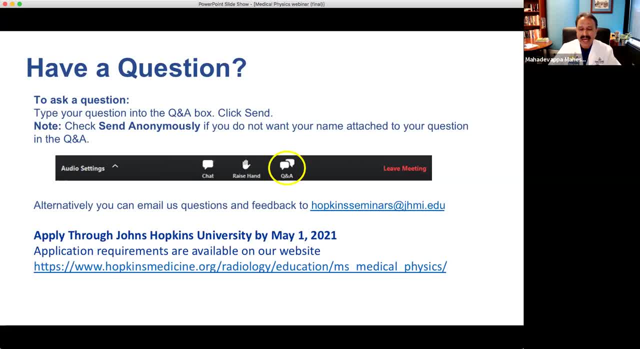 to nuclear physics background, so they're leading into it. I would also advise, if you're- whoever- the undergraduate, if you are in your undergraduate, look for program for a summer opportunities, because our professional society, American Association of Physicists in Medicine, offer a summer program, a summer program. 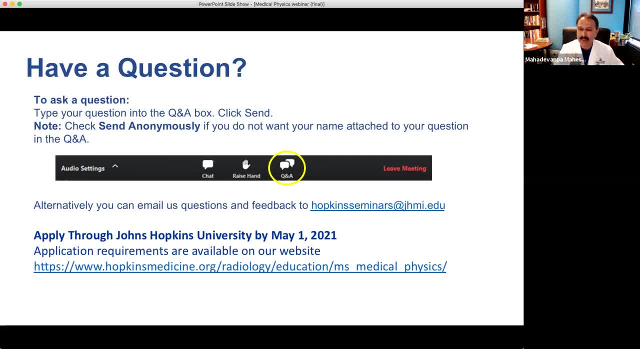 a summer scholarship for interested students to apply and they will place them in different research lab, in medical physics lab, so they can expose to the medical physics for six to eight weeks, which is also it also includes scholarship. So I would direct any of the students to also visit the American Association of Physicists. 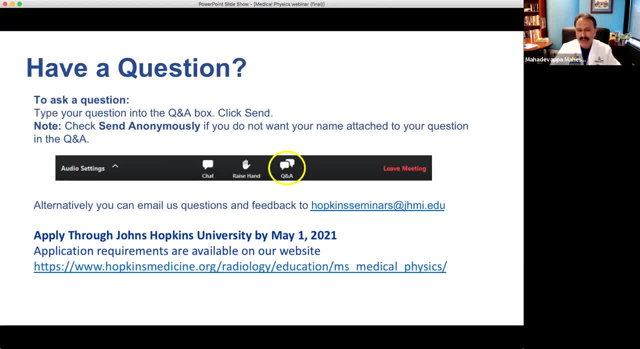 in Medicine website aapmorg. it has a lot of information, especially the summer program where the AAPM also offer one-fifth One for the, a program called DREAM program for diversity of inclusion research program. Again, these are like six-week summer program for anybody interested in this area should. 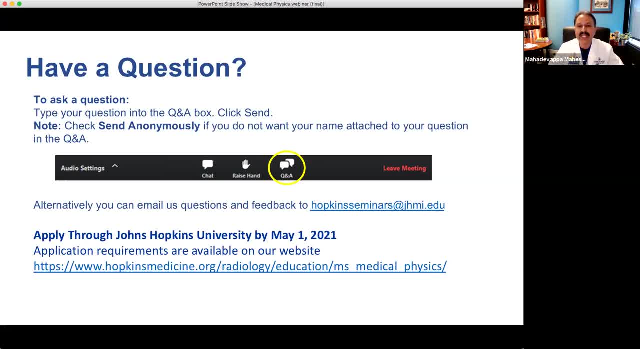 consider exploring this so that they'll be introduced to the program, get a pathway what medical physics is all about, And if you have further question, you're welcome to email to the program and we'll be happy to answer those things. Thank you. 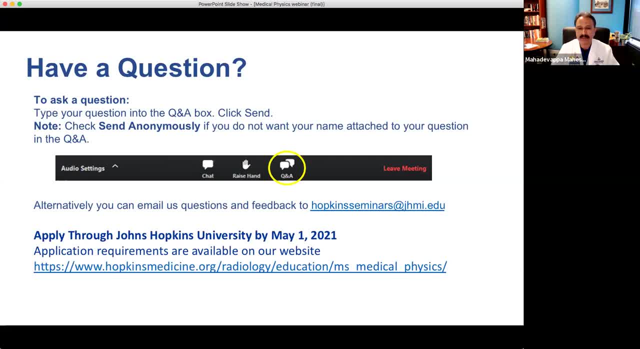 Any more more, more directed questions. So just just to add a little bit to that. I see there was a question about a nuclear medicine BSc degree, whether that qualifies. I would say a couple of things. if, if you've had as part of that, if you've had the physics, 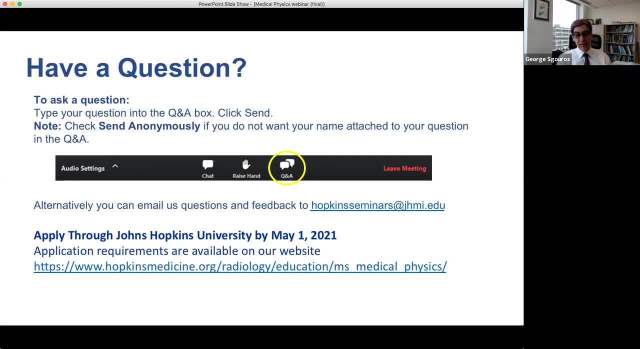 and the math, then absolutely. The other thing I would add is: don't neglect biology, that's, you know there's a medical component to the physics- that you would be doing. So, to the extent that you can learn as much as you can about biology and medicine, that 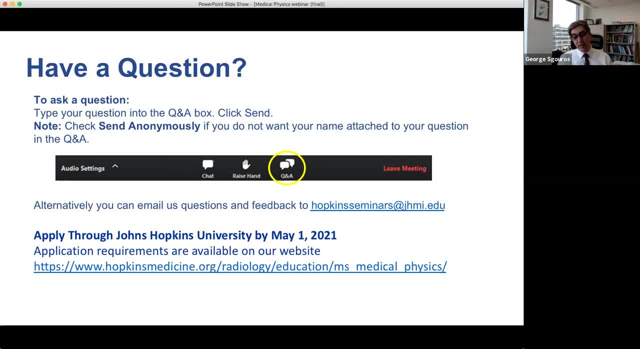 will sort of help, kind of make you unique and and frankly, we're looking for individuals that that have a certain level of diversity. So if you enjoy poetry, please highlight that, as long as you have the fundamentals. So we're not looking for straight physicists, we're looking for people that can enrich our 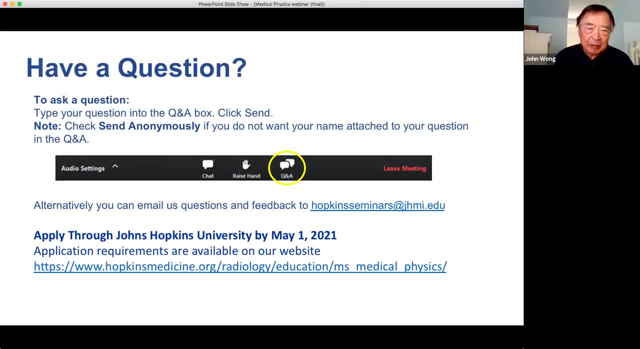 community. Yeah, Let me just modify my, my, my comments, Okay, Okay, Thank you. My my comments earlier. There's no strict requirement of what physics level of physics that you need to be a medical physicist. You have to be. you have to have physics knowledge, some math knowledge. 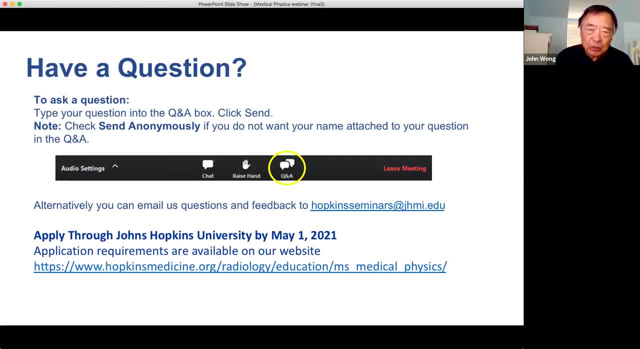 Okay, But just remember that you are the person that's going to be communicating with our partner medical physicians. So we we need to have an understanding of the physics of the technology Or the therapy techniques that we use so we can convey and work with the physicians. 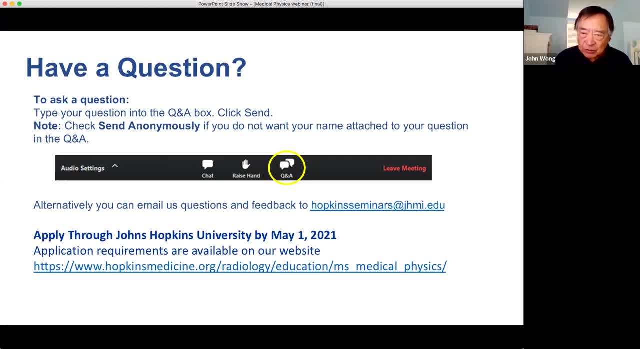 That's roughly the level of physics you, you, you have to master. Okay To, to be a medical physicist. Another another highlight of our master's program is this is not based in a far away university where you don't have contact to the hospital. 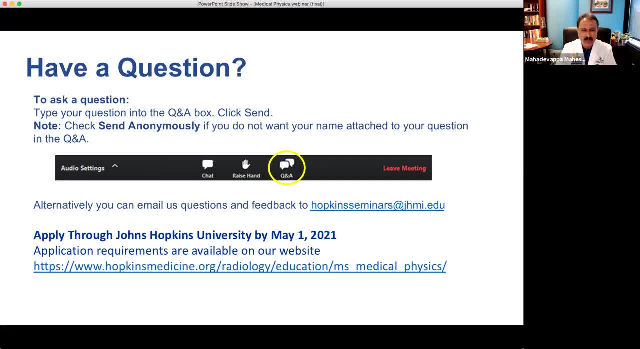 We are based in the hospital, in the radiology department, Which means the student is get to it And, as a nurse, we are told to communicate with the physicians and the physicians are told to communicate with the physicians, And you have to be very specific with the physicians and the physicians and the physicians. 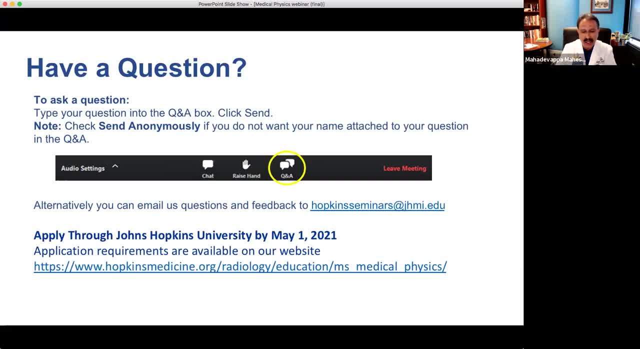 to be able to communicate with the physicians, And we can do that, So we are focused on a daily basis What the clinic is all about, And that's how I was trained back when I was doing my doctor studies in the hospital. that 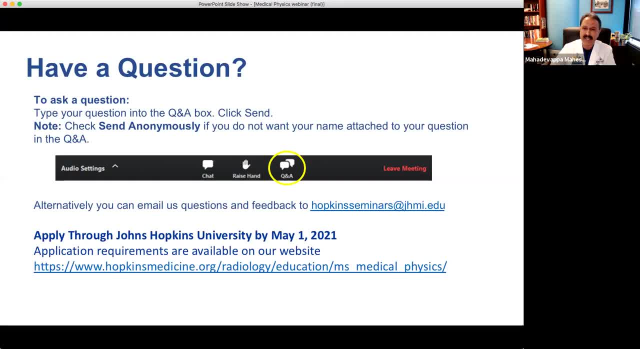 gave me a lot of wide perspective what medical physicists do on a daily basis. In addition, we'll also learn how to communicate the physics aspect with nonphysicist And- that's also equally important for a medical physicist- with our physicians, with the technologies. 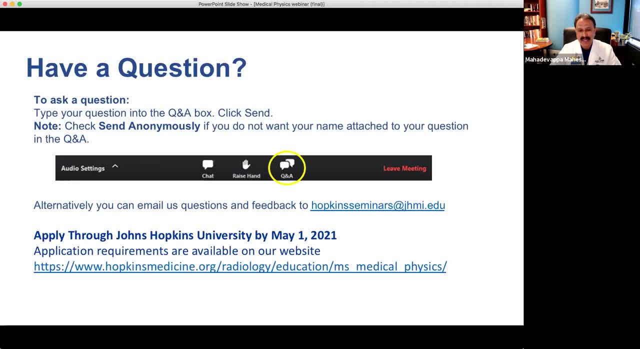 and the nurses. So that's what we are aiming to: develop a wholesome program And, as our director said, we are interested in struggling with the physical aspects and, as our director said, we are interested in students. who is a wholesome student, not just one? 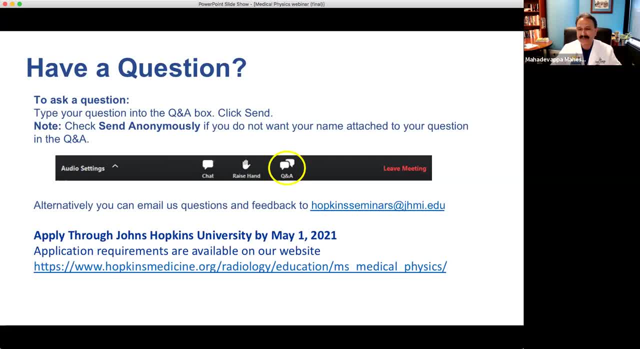 one focus, like he's also interested in other things. perfect, so another question we received was that from sarah um. she says i noticed that power plants was listed under industry for possible career options. could you expand more on this? how does medical physics play a role in a power plant? can you elaborate on that? yes, absolutely so. the direct. 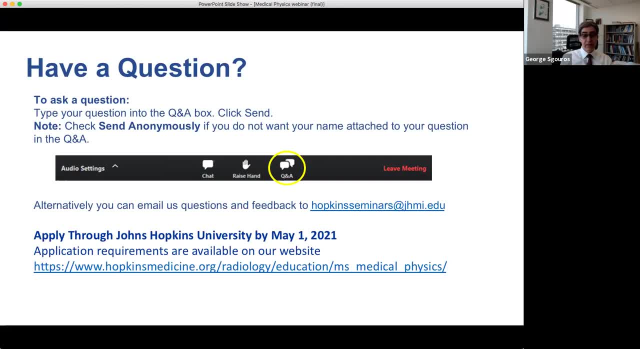 answer is sort of as radiation safety officer, but i'd like to expand on that. a medical physics background really gives you an opportunity to work in a wide variety of industries. uh, nuclear power plants are one area you can think of. uh, manufacturers of medical equipment, manufacturers of mri machines- uh, a huge diversity. 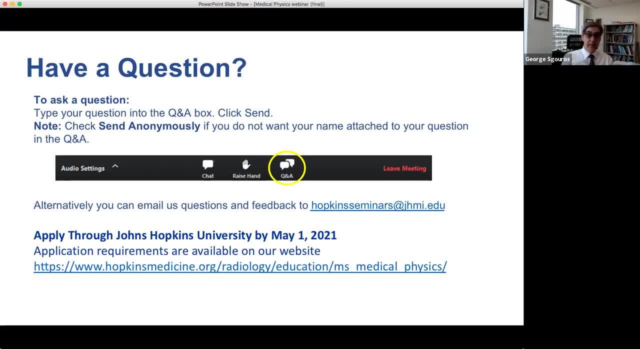 of potential uh areas that one could work in, and to some extent it depends on how, what direction you you find yourself most interested in. uh. the program is focused on medical physics uh, and the direct link to a power plant would be in terms of radiation safety. so that's that's where, that's why the power plants are listed there. pretty much any scenario where 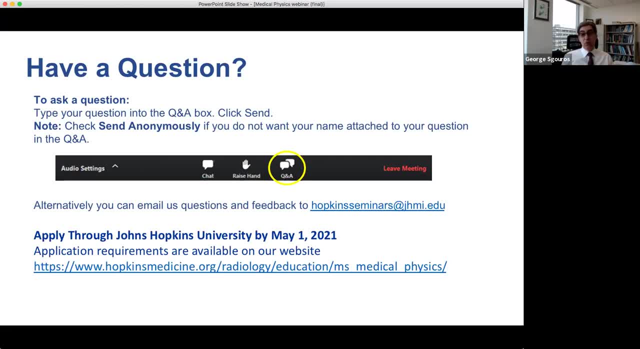 where, where in a, in a, in a in any setting, people are working on a power plant, they're working on a power plant. they're working on a power plant working with radiation or radioactivity, you will need a radiation safety officer. so so one of the areas that might be interesting to the applicant is that we work with nasa too. okay, absolutely. 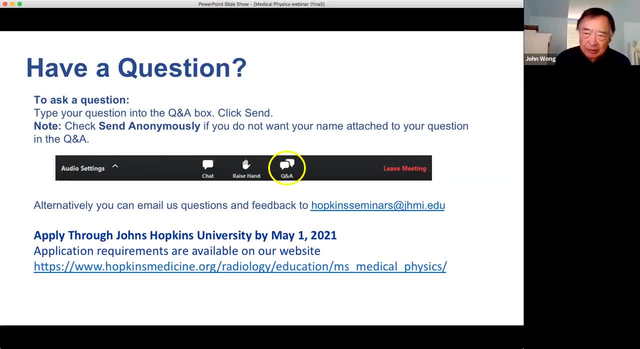 many of the space flight and uh radiation that these astronauts are receiving has become a a very interesting uh uh, an applied medical physics uh uh topic. okay, so why for rsd of uh of profession? so we also have a lot of questions here about if whether we are going to be getting the camp. 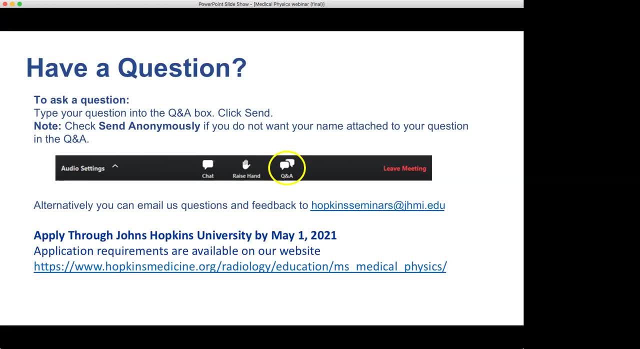 pep accreditation soon. yeah, i'll answer that. yes, we are, you know, processing apply for the king pump accreditation and we are expected to get the credit before the fall semester. thank you, so i let me, let me, uh, interject too. is that the campaign accreditation is retroactive? okay, so why? 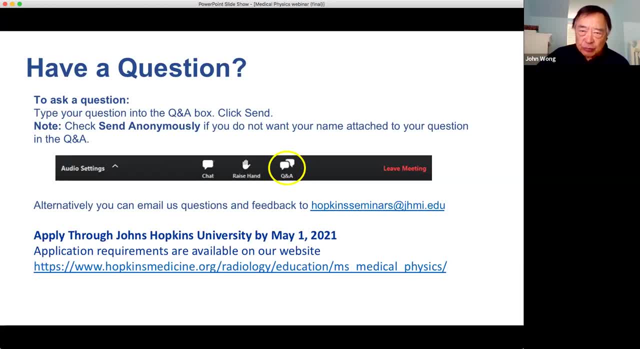 in the process of acquiring formal accreditation. uh, if, if we have shown our intent or we have started the process in the accreditation, anyone that get uh is admitted to the program now. okay, uh will be. can can see that they come from accredited camp. accredited medical physics program. 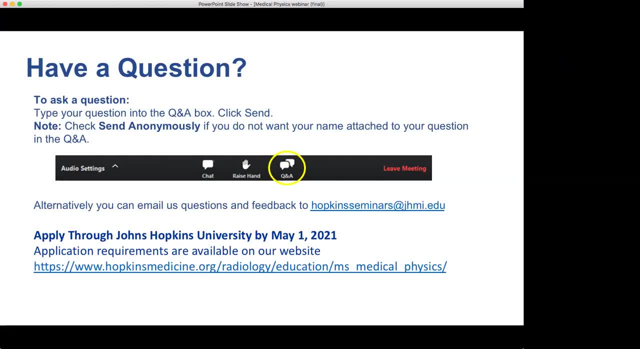 great. we also have a few questions related to the type of program that is used, such as python. so can you elaborate on the programming language that is most used by medical physicists? uh, absolutely so. uh, you know, i think it depends on on your generation and where you 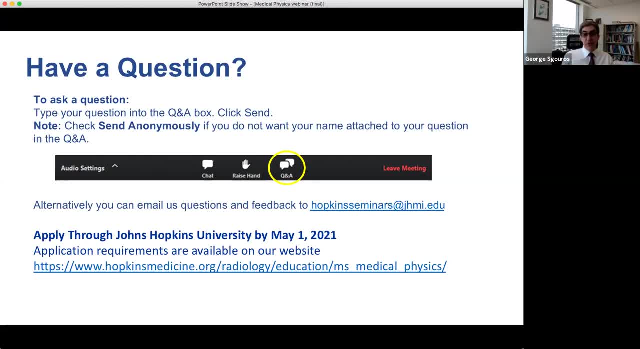 sort of. so you know, python is is very common. if you're doing research in particular, i know that young uh uh is using it. it's it's one of the more popular languages in in our research side of the division uh, tremendously versatile and powerful. i sort of grew up with fortran uh, but but i so so. 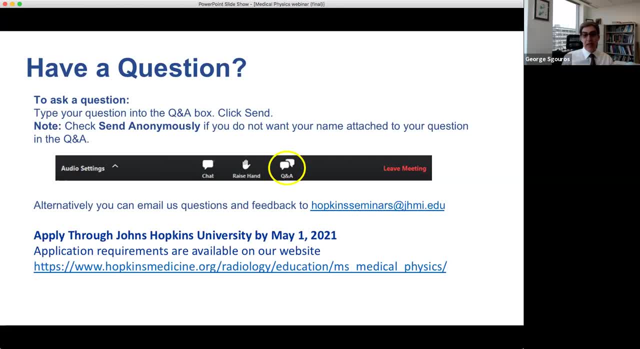 if you understand programming, i think you can pick up these these different languages quite well. if, if you have the opportunity to learn learn python, definitely do it. it's something i plan on doing at some point when i get some free time- great. we also have a question around the completion time for the program. 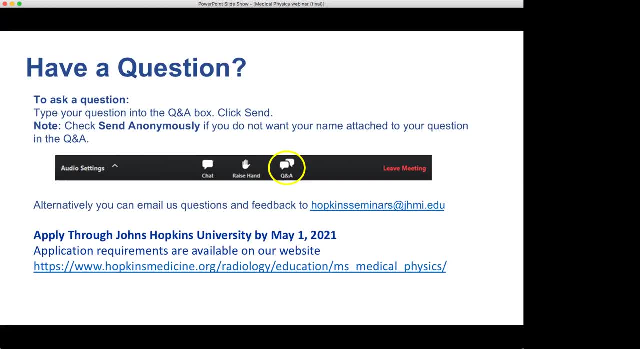 is it a two-year completion? does that include the thesis route or the non-thesis route? so yes, it's a two-year program and the and it includes a thesis. so the thesis is based on the research done during that summer. to elaborate a bit more on that, as you're attending classes, 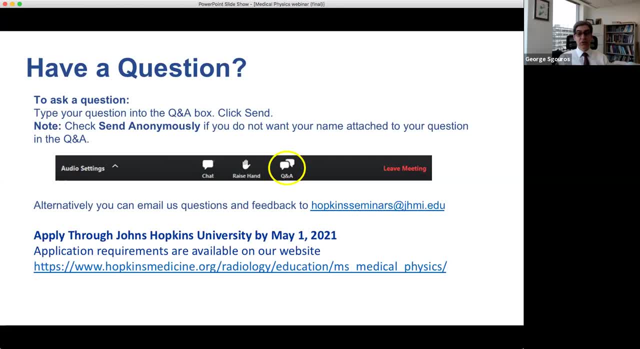 you'll hear seminars, you'll see different individuals within hopkins and they'll explain what they do for their research and you'll have an opportunity to select someone to do your research with. and that really forms the basis of whether the thesis would thesis write-up would constitute. 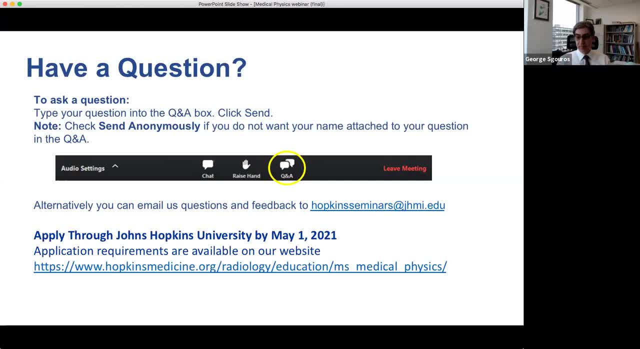 anybody else want to weigh in on that. i think that you have. you have clearly said that, and i just want to add on to the point that, given the wide of variety of faculty exports here, finding a thesis topic that can fit for this one is not a difficult. it will not be a difficult one because we have a very intense research researchers. 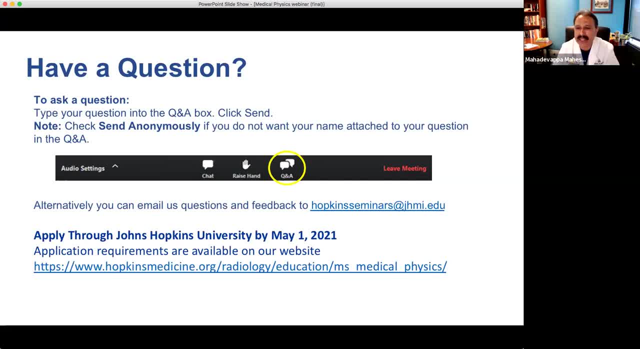 here and you'll find very interesting medical physics related topic for doing any thesis great. we also have some questions around whether classes will be in person, given COVID-19, and is remote access an option? Can you elaborate on that? You know, I mean, I wish we had a definitive. 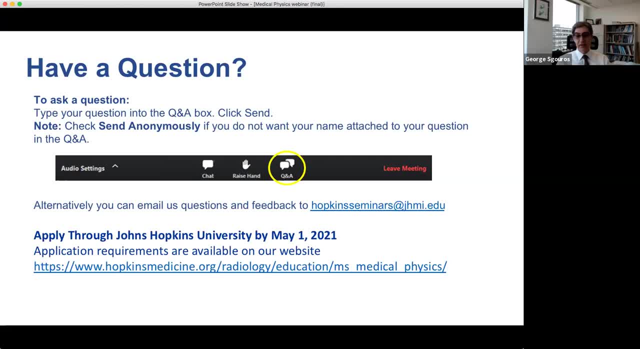 answer. We're going to go by state and school of medicine guidelines. We're currently in phase one And I know we all sort of want to get past this. At the moment it's hard to predict the future. We really all wish we could. I would love to have us do this. 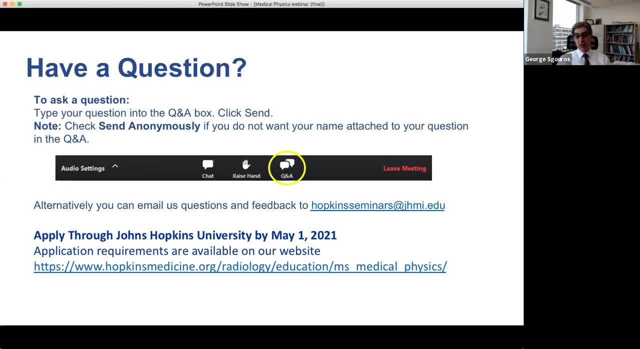 all in person. But if we have to, we're certainly prepared to do it online. But right now the university as such is also exploring for the fall semester to be in person. They're exploring again And most probably it may be going the direction, but in-person. 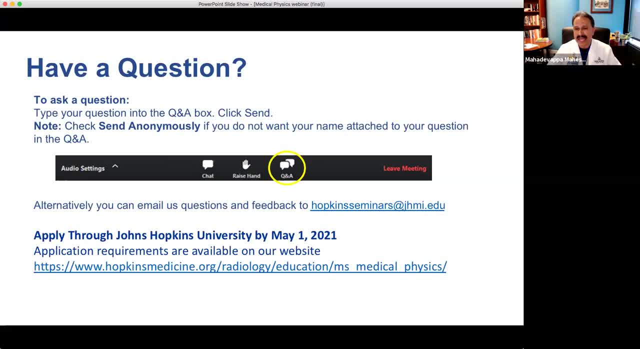 class would be what I would prefer in the sense because the students will have an enriched environment to learn. Especially the practical medical physics is kind of nice. You just have to see and learn and interact and learn. So that is our intention, So we'll go by the university policy. 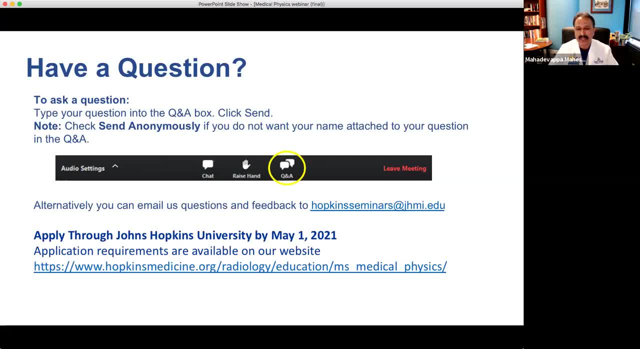 but most probably it's looking in the direction of having in-person class. Yeah, And I think, to the extent that we can be socially distant and follow all the rules, I mean it's certainly a possibility, No guarantees. It depends a lot on how we all behave with masking and distancing and doing all the things. 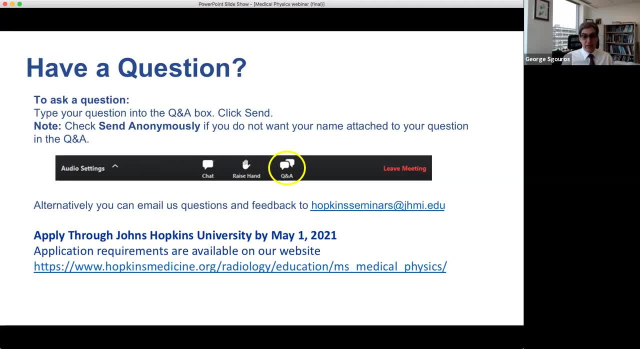 that are recommended to help get us past this terrible pandemic. We also have a lot of questions around for college students pursuing their bachelor's degree and what they should be pursuing in college levels such as biology, And I think that's a good question. I think that's a good question. I think that's a good question. 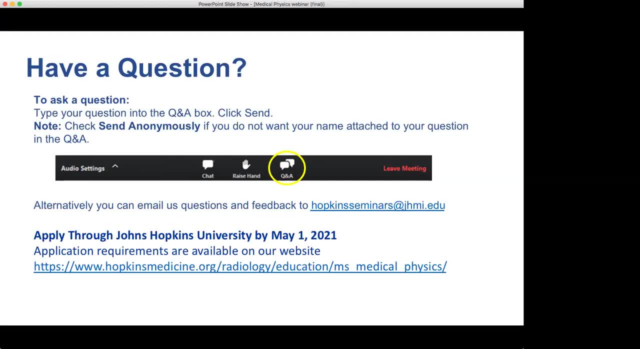 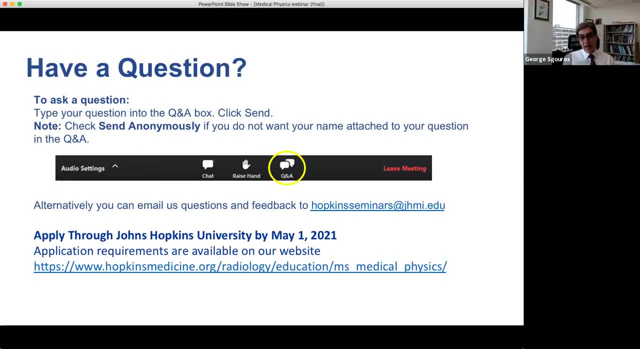 Yeah, So certainly physics and math, And if you have interest in biology and anatomy, those are enhanced. But fundamentally we really need to have students that understand the physics, are good at math and potentially at the level of differential equations, mostly because that will make them better medical physicists. uh, you know, as doctor, as as dr wong, 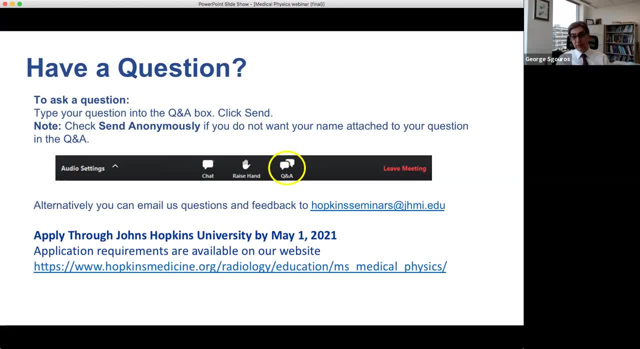 pointed out. fundamentally, the job is really interacting with physicians, to some extent with patients, uh, but you really need that physics background. uh, and the math background are going to be very helpful as, as you go through the coursework and um want to become a successful, uh, medical physicist, let me let me interject and advise to students who are an undergrad. 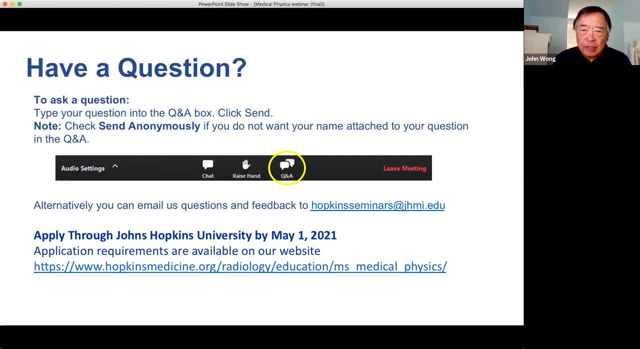 want to get into medical physics, you don't have to do it at the undergraduate level. uh, you have to be able to by the time you graduate from this accredited campus. accredited medical physics program. six core, depending on the discipline you have. there's six core, uh, let's say qualification you. 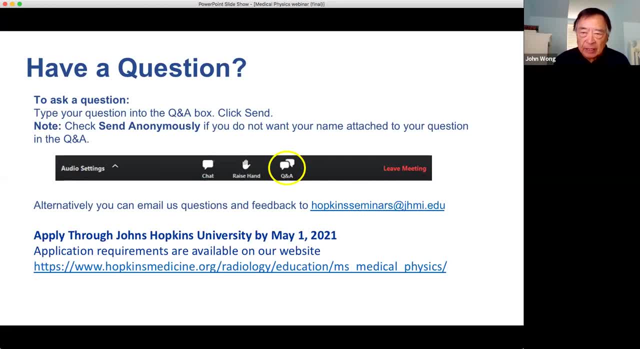 need to go into professional training, that is, if you want to practice as a licensed or a board certified medical physicist, you have to go through residency like the like the physicians. at that stage, though, uh, you will see the qualification you need uh to be accepted in that program. 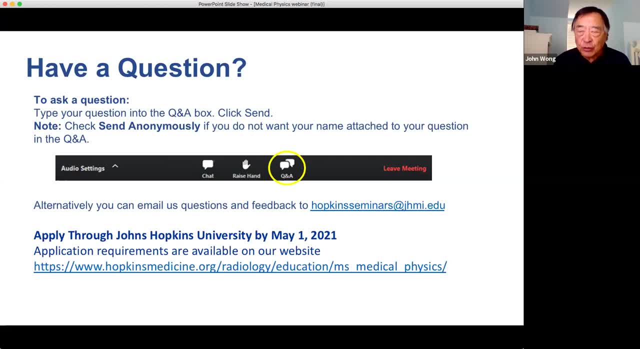 so anatomy is one of them. uh, radiation biology for therapy, physics radiation biology- is one another one of them. so i believe the six core training that you need to have and you can visit the aapm website for more information. okay, i, i just want to emphasize: when you get into medical 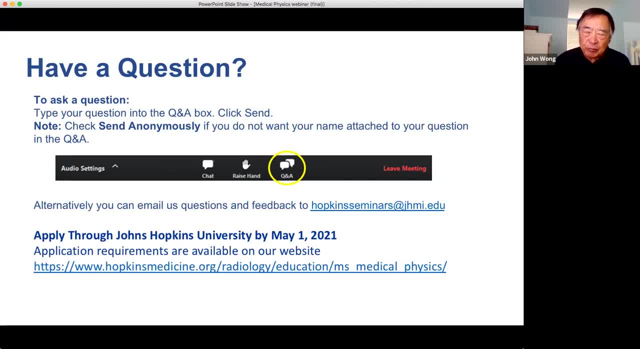 physics, uh is a very committed but very rewarding profession, because we are the parallel counterpart of the medical doctors. okay, so that, and that's why we have now both certification in our professions too. thank you, can you also elaborate on what you look for and expecting candidates uh? 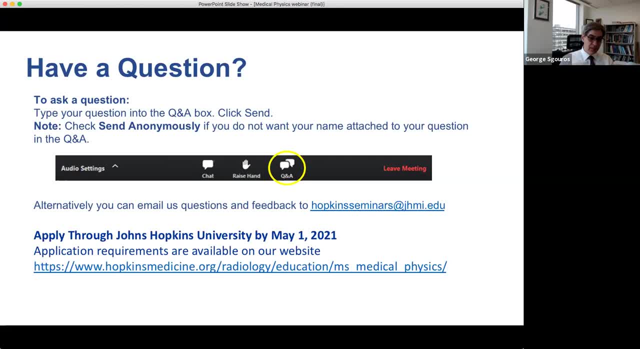 you know, we look for for uh uh dynamic individuals that have the right background and are really interested in the career in medical physics. uh, we also, as i noted early on, we want to increase the level of diversity in medical physics. so, uh, that'll be part of the decision process, you know. basically, it's, it's sort. 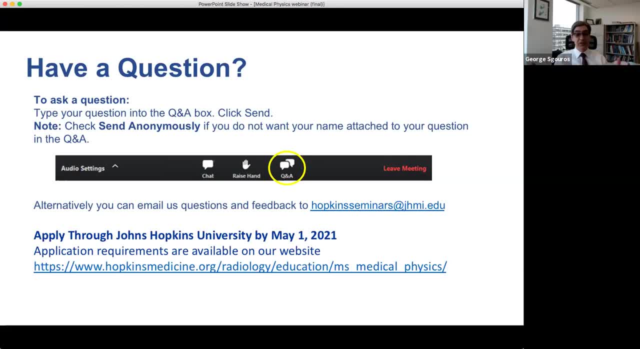 of quote unquote, a holistic thing. we look at the total individual uh and then kind of make an assessment and then we look at the overall situation and then we will then consider it as part of the on whether they'll benefit from entering the program and to what extent they'll help the. 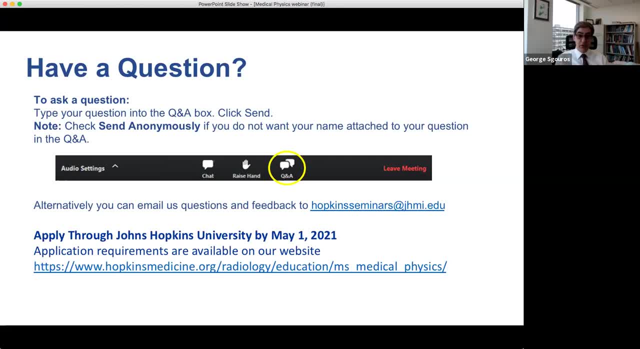 field and be successful. These are really the fundamental metrics that we'll use. You know, other than that, I think- and you know we've talked about the requirements- but goes back to sort of the philosophy: We're looking for individuals. that 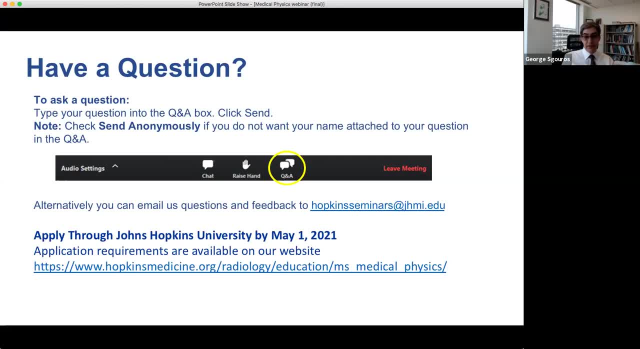 recognize that this is a valuable thing. It'll benefit them long-term and it'll benefit the field, I think also. just to add on: the letter of recommendation also makes an impression because we want to hear what others have been telling about you. 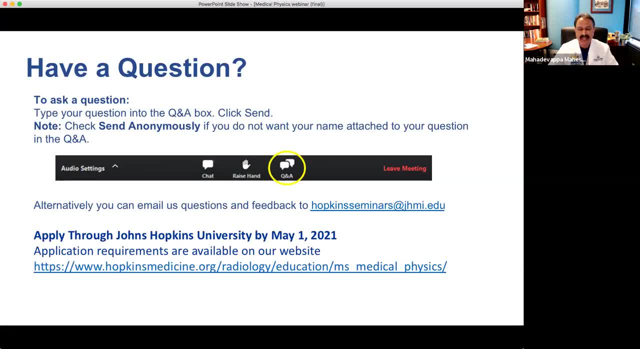 So having a good recommendation letter is a plus sign for any candidate for any program, So I would advise that one. So I want to give you an anecdotal history here When I first started. there's no such thing as medical physicians. We all found a path. And if you talk to all of us here on this panel, 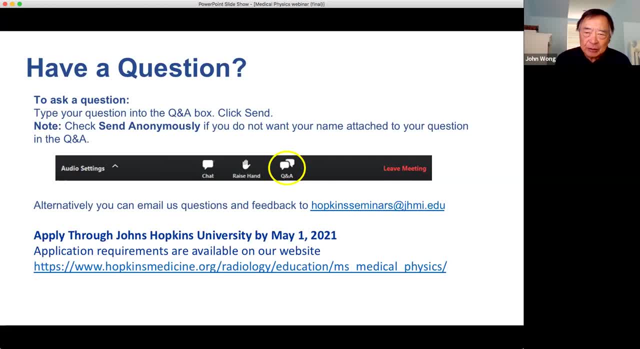 there's something about us really liking to deal with healthcare patients and applying physics knowledge to medicine. Okay, So you have to think about: do you like working with patients, You like working with healthcare problem, And then also, are you passionate about it? 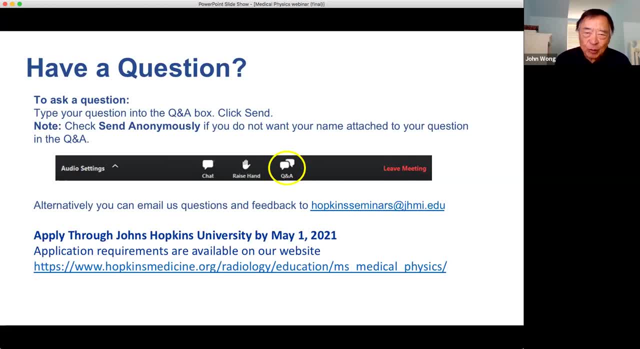 Because you're going to make this a worthwhile profession. So if I'm looking for someone who wants to come to our program, I think the most important part is commitment and passion. Yeah, Just to add a little bit more about my background: I actually started by working in. 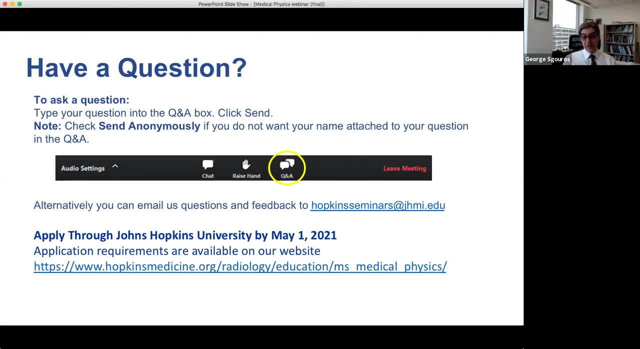 the lab as a high school student and started in physics background undergrad Okay, But then over time I found myself more and more interested in biology. That's why my lab is doing research And you'll find that it's heavily influenced by the biology. I'm understanding. 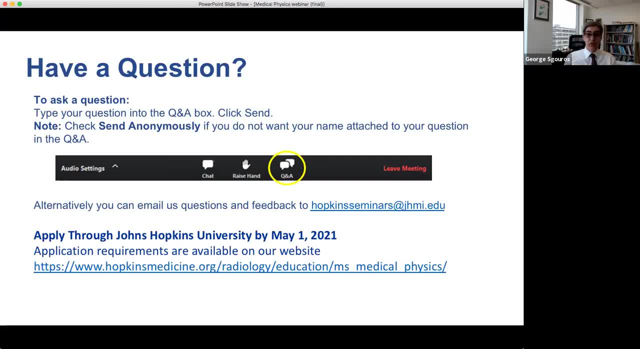 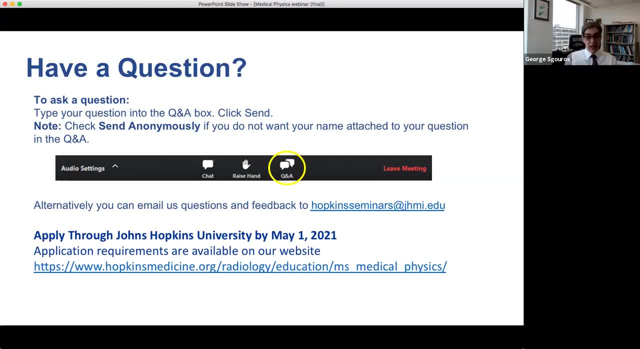 And sort of an interest in both the biology and the physics, and medicine as well, And also the other aspect of medical physics is for those who are practicing in pure physics. medical physics is a very applied knowledge And you can see the difference in a short time. For 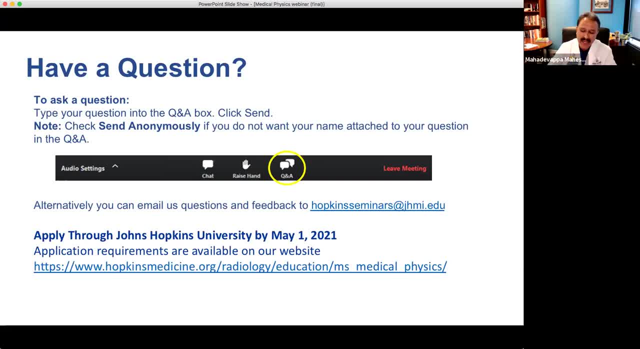 example, if a patient or somebody is concerned had a CT and they're worried about radiation dose, let's say, and they have read an article about radiation dose and they're concerned. And when they approach a medical physicist and we are able to answer, and convincingly, they're. 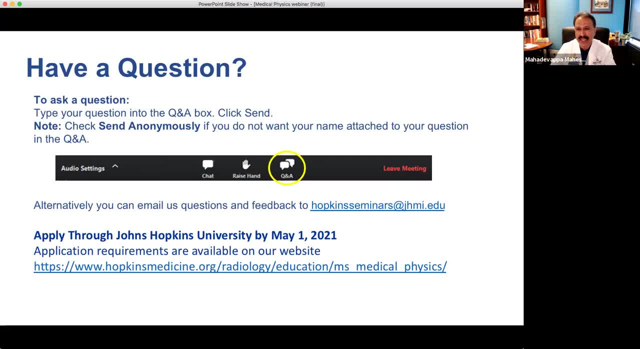 telling them what are the plus and minuses and why they should get that particular imaging. that gives you a fulfilling sense of being in the field, because you are working along with the physicians and trying to help as a team player in the healthcare setup, Not only financially. 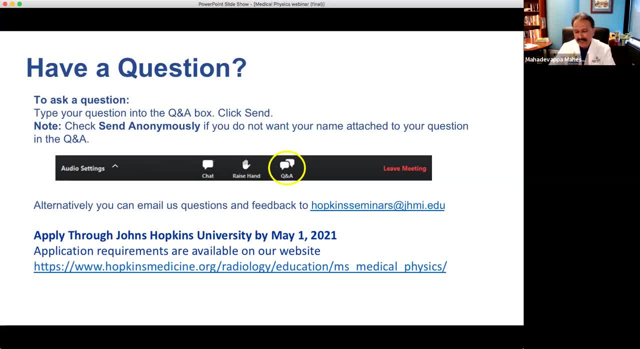 but in a broader sense, because you have to work with the healthcare system as well, Not only because you have a good job, but on a regular basis. your interaction also makes you feel that you're contributing to the overall healthcare set in the positive direction. 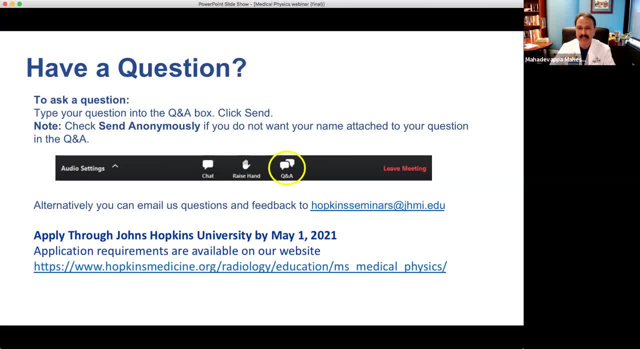 And I feel that to be very advantageous of being in the field. Thanks, Dr Mahesh. We also have a question around the clinical experience Students will experience in the program. I know we touched on that a little bit. Can you expand? 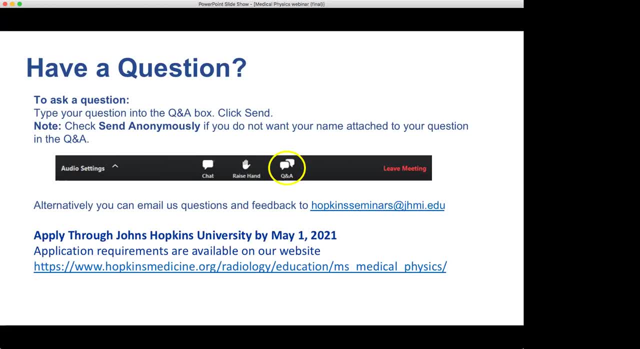 on some of the things that students will experience from a clinical side. So I can take that question because, like right now, so my role, one of the role in the hospital, is try to make sure all our imaging modality are tested annually and also meet all the regulatory. 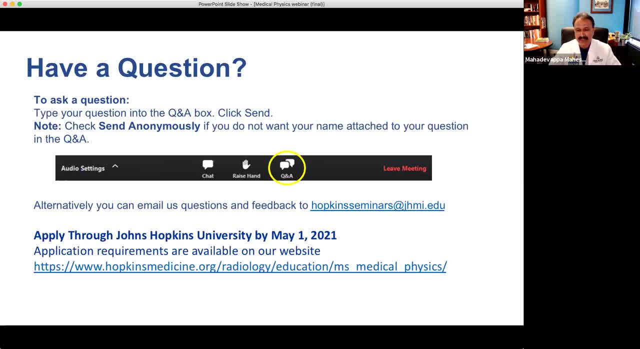 requirement. That means we want, we test that on. for a quality control. We need people, We need so we can really offer the students an opportunity to do that. We can really offer the students an opportunity to learn some of these quality control aspect like accreditation requirement or a. 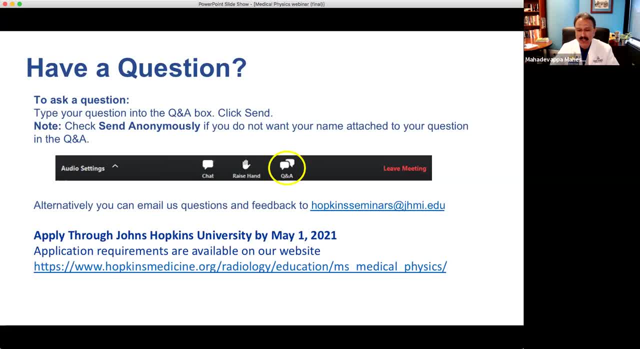 hands-on experience because, Hopkins, we have such a wide variety of imaging modality. to just to give you a stat, We have 22 CT scanners on campus, about 20, more than 20 MR scanners and we have totaled about 150 X-ray tubes in diagnostic imaging alone. So we have such a wide variety of 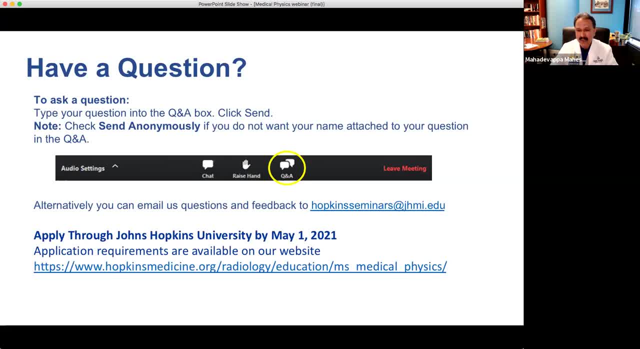 rooms and I kind of assure you that the students will be exposed to clinical experience so that that will put them in a good advantage when they apply for residency or anything after the master's program, if they want to pursue the clinical medical physics board exam and so forth. 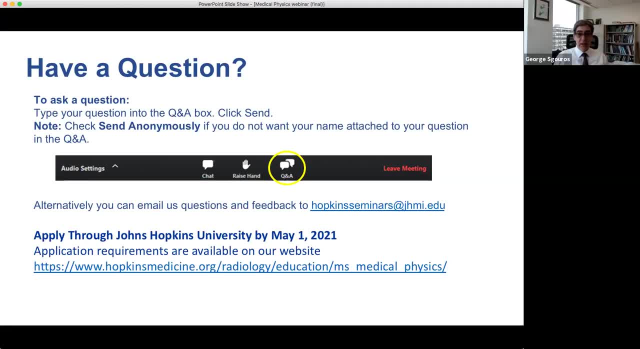 Yong, do you want to add to that on the Luke Med side? Yes, I just want to add that, And then we'll get to Dr Wang. Yes, Clinical rotation actually required on offer, the required curriculum, So you will definitely have the experience to get the first. 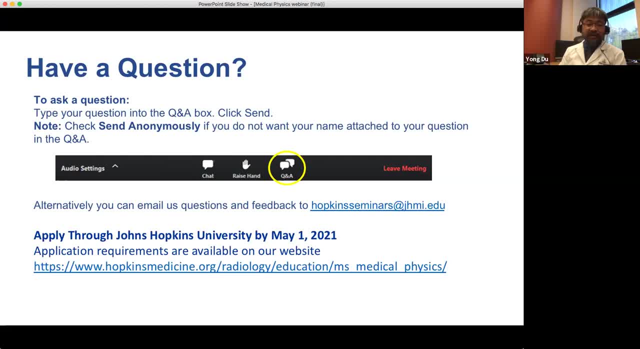 hand experience in the clinical medical science And then we'll get to Dr Wang. If there's a lot of expertise in the clinic, talking with you, know technicians, physicians and the physicists, to see how they apply those techniques in the clinic, how to use for. 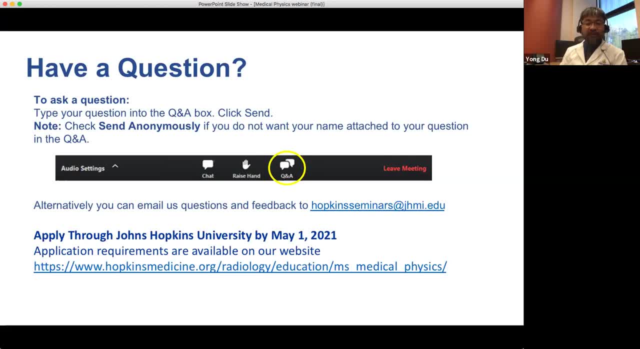 diagnosing and treating patients. Yep, they're definitely going to have a lot of experience here. Dr Wang, are you on the line? So one of the major knowledge that we have acquired in therapy, medical physics, is the interaction or radiation with matter interference: radiation by material. to measure radiation: into each and every one of our participants. So, in addition, we can now provide the methối irmi polutcíaandi cube physiotherapy unbelievably undoubted. Doctor Wang, your 1970s was an amazinggga. 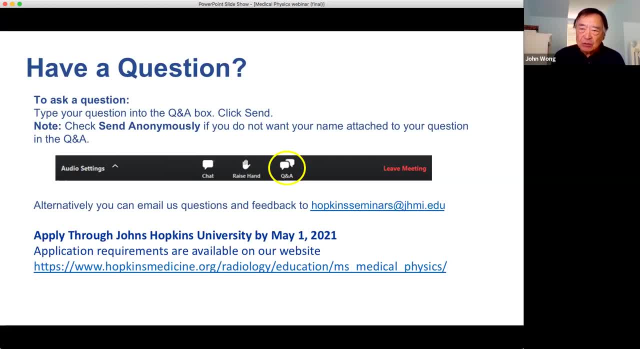 You know from that, I'm pretty sure that everyone should have been getting the right hardships from the good example Gh Xinqing curiosity about the second family right before radiation with human. So the student going through here will have a chance to go through the. 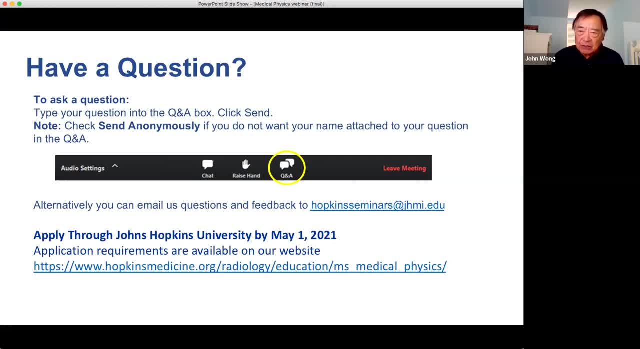 imaging component where we understand the problem that we have to treat and then we deal with the optimization of treatment on a computer model and then also participate in the setup of the patient to go along with the therapists, that you can see how the patient is set up to receive the dose and 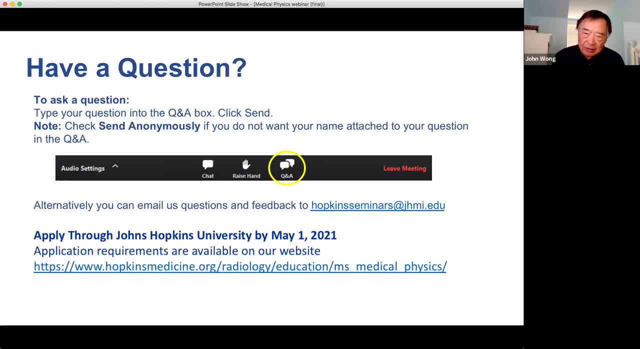 then we go on and need to verify that we did it right. So that's the very intimate interaction with the clinical care of the patient. Best opportunity you have in the therapy physics part of this course, Great. I think we have time for just a couple more questions, So another question. 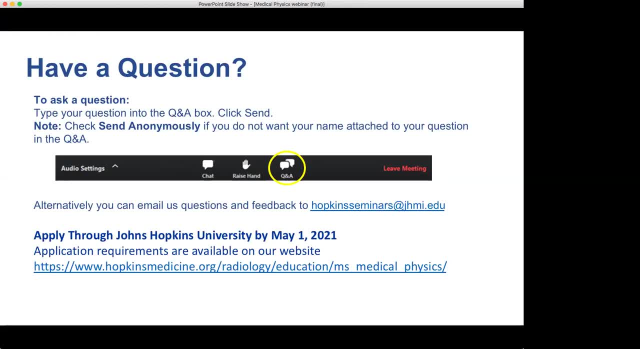 we received was: how large do you anticipate your entering class to be and how many applicants will you accept? So we're starting out. we're going to accept five or five to seven applicants initially. So we're sort of not starting very big for a master's program in medical physics. 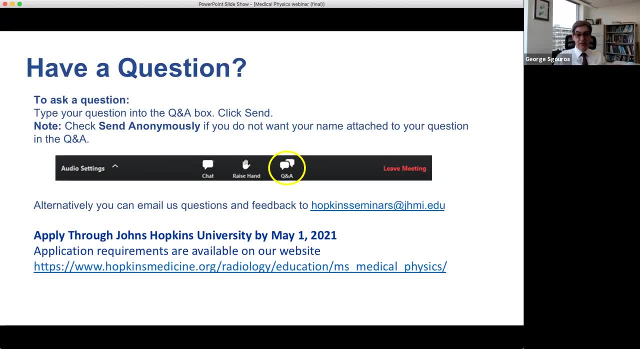 I think Dr Du can talk about to some extent typical class sizes in in these kinds of programs They're not particularly big. Go ahead, Yong. Yes, we are hoping to have five students starting in the first master's. So you know, based on how many applicants there is, we may you know. 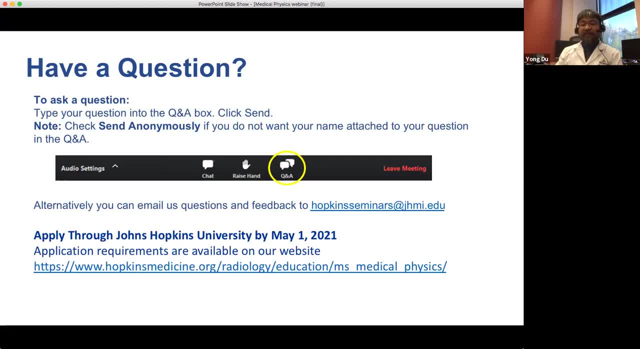 give offer to maybe 10-15 people and usually, based on our experience from other programs, usually now one-third or one-fourth people will come. So that's the our target. so basically five students start the class. Great, Also for students that would need to relocate. can you expand on the housing costs in Baltimore and the housing options? 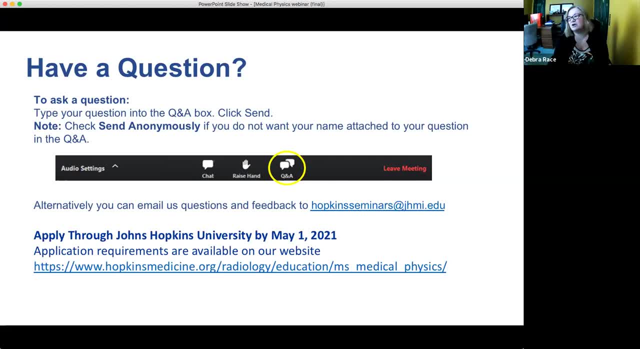 So okay, go ahead. Yeah, okay. so naturally the cost will vary on you know where, where students live, or you know, and what type of accommodations they want. I think they typically start out from like $1,000 going up. The nice thing is is that the School of Medicine has a 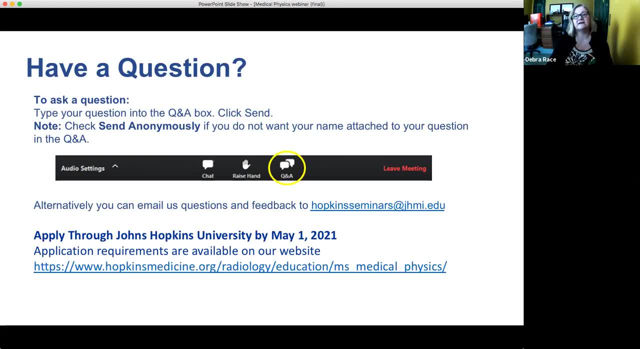 great off-campus housing website that has like an interactive list listing and it it breaks down properties. It can put you in touch with roommates. They have like a like a buy south furniture kind of page. So that's we usually tell students to to stay in the home. 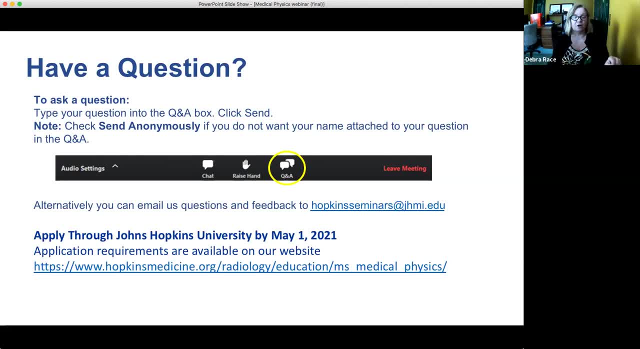 You know students to start with them, because you can put in. you know like how much you want to pay. You can put in like this is the least I want to pay, This is the most I can pay, and then it brings up all the housing that's available. I will say that where the medical campus is is located, there's. 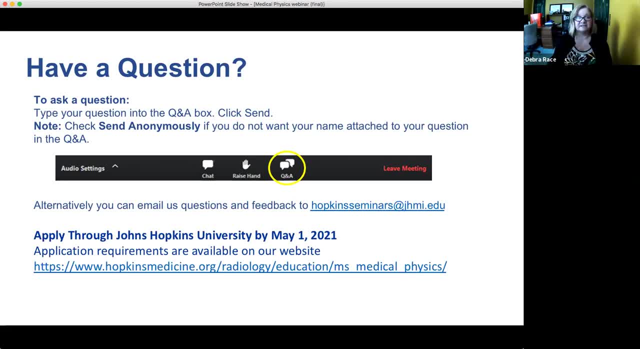 not a lot of housing. So what typically happens is is: the university undergraduate campus is about seven miles north of the medical campus, and Hopkins has a shuttle service that runs from both of these campuses all day, into the middle of the night, and most of the students that are 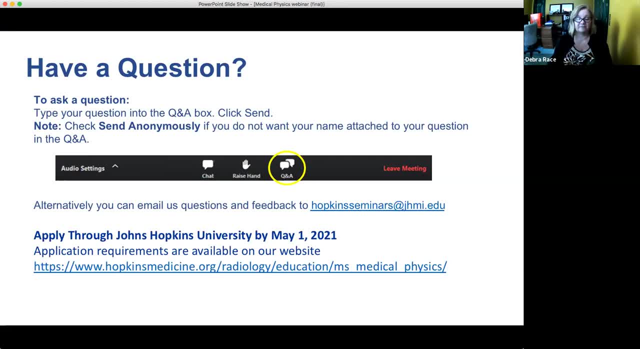 actually in either the School of Medicine, the School of Nursing or Public Health. down here at the medical campus they live up by the undergraduate campus because Hopkins, even there, does not offer any housing. It's all commercial off-campus housing, but it's plentiful. and again, the website. 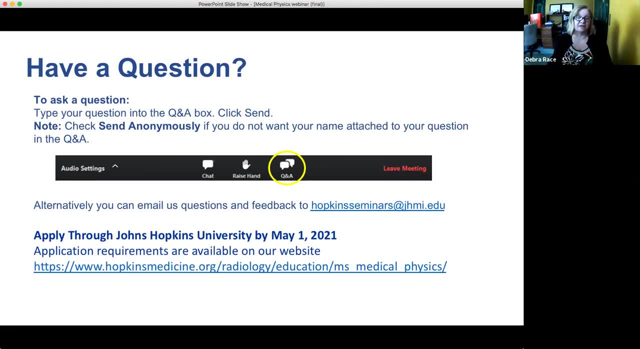 is really great, and if you, you know, if you can't find that, send us an email. we can point you in that direction. Yeah, I would. I would add that that I walk to work, so so there are some really nice places near the, near the water, near Fells Point, that that one can look at. They're probably 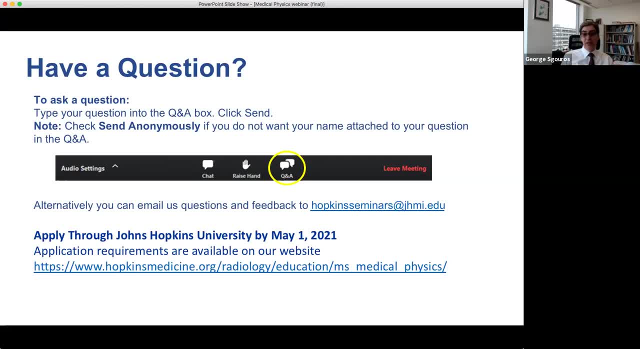 depending on your budget, a bit more on the pricey side and there are shuttles to many neighborhoods in the surrounding neighborhood. So it's a Baltimore is actually a wonderful place to live And I highly recommend it. We moved from the suburbs to to the city and I enjoy walking to. 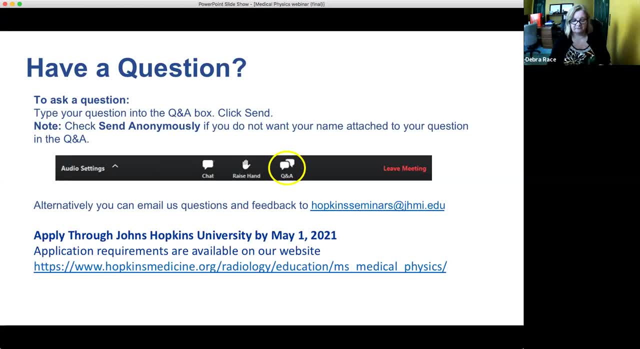 work every day. I'd like to clarify something that was brought to my attention. The actual deadline for the application submission is April 15th. I think the slide that shows questions says May 1st, but it's actually April 15th.